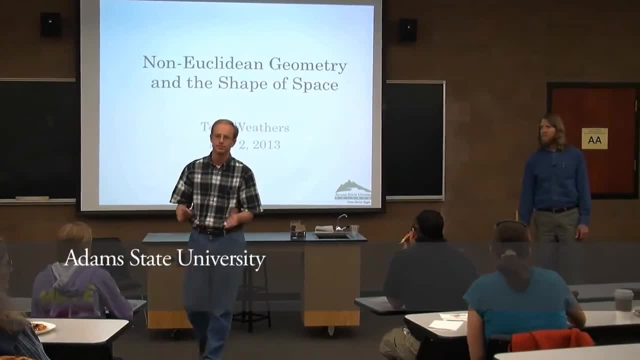 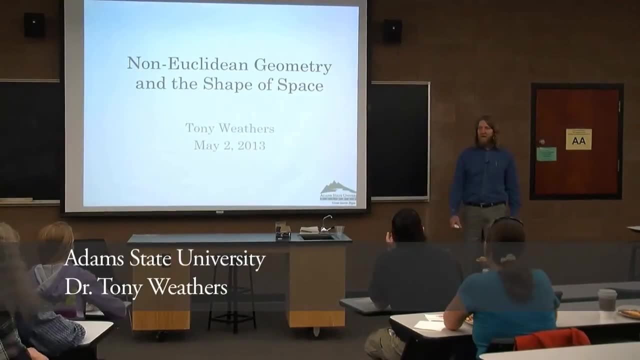 And it's my pleasure to introduce Dr Tony Weathers from the math program. Alright, thank you all for coming and let's get started. Today, as you see, I'm going to be talking about non-Euclidean geometry and the shape of space. 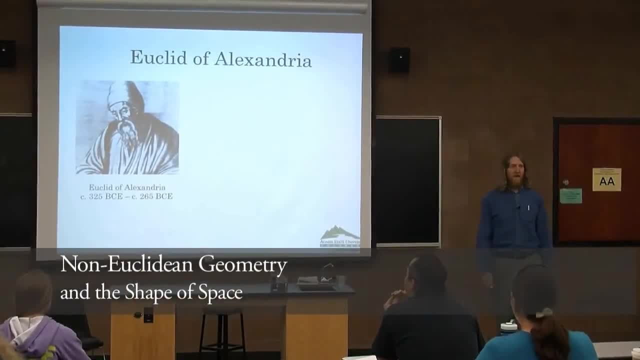 And so we get started. We first need to talk about Euclid. Now, you've all heard of Euclid and this is kind of interesting. I pulled this picture off of a website- I'll give you the address of later- a history of math webpage. 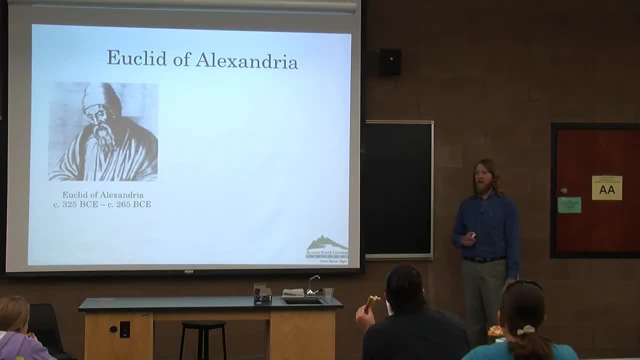 And I can't imagine any possible way that that's anywhere near correct. I mean, Euclid lived 2,500 years ago. How on earth would anybody know what he looks like? Well, the country of Greece issued a postage stamp in his honor some years ago. 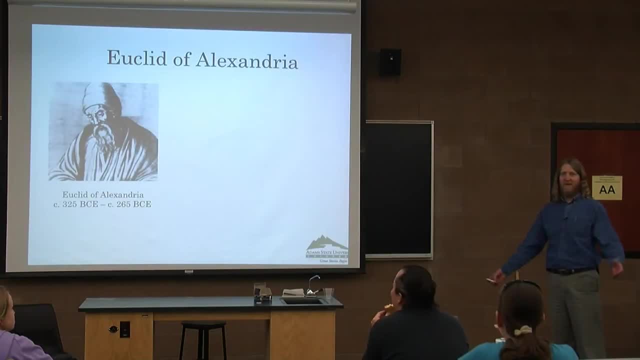 And well, you've got to have a picture, right. So maybe they just made it, They made something up so that they could make a picture of him anyway. So maybe that's what he looked like, maybe not. We don't know a whole lot about him. 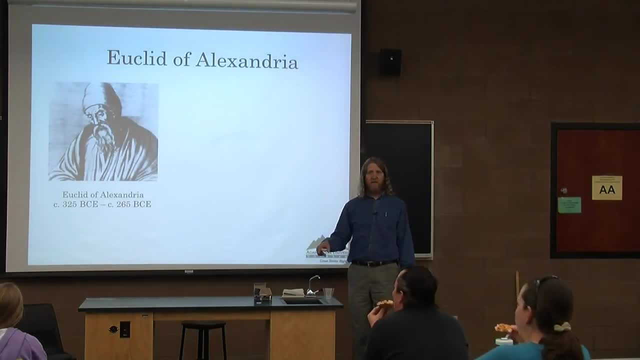 We do know that he was writing, was active around the third 300 BC And they've sort of pieced together that he was probably born around 325 BC, Lived to be about 60, which was a pretty notable accomplishment back then. 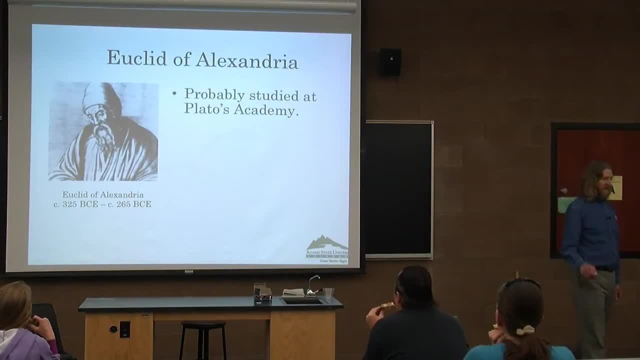 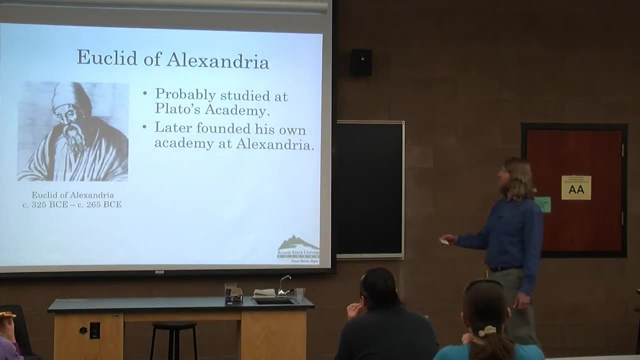 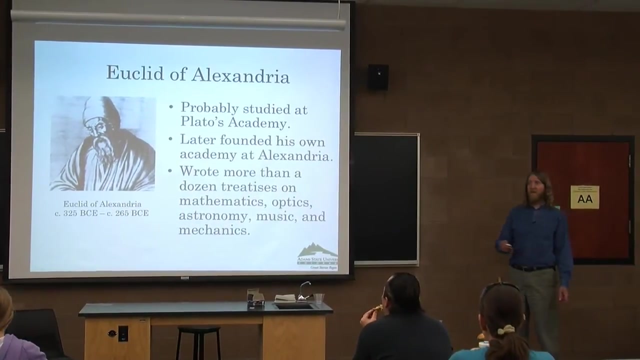 He probably studied at Plato's Academy. He at least studied with some students of Plato's Academy, They're pretty certain of that. He later founded his own academy in Alexandria And wrote quite a bit, Wrote more than a dozen treatises on a variety of topics, including mathematics, but also optics, astronomy, music and mechanics. 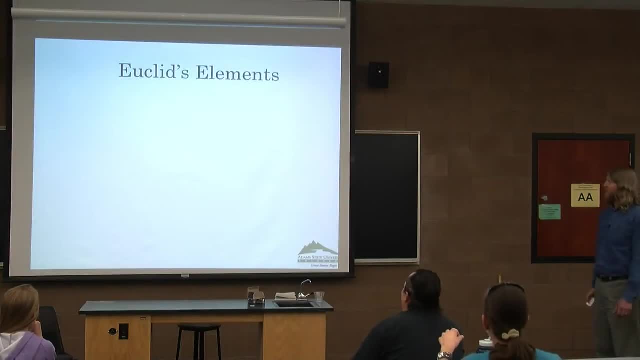 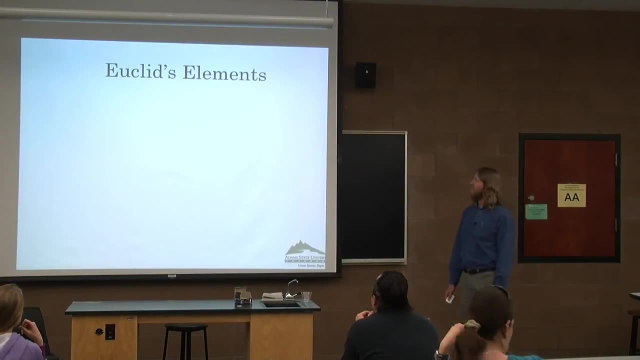 Of course, he's most famous for one particular treatise that he wrote called His Elements- The Elements of Mathematics. really is what it was about. It's mostly about geometry. It's 13 volumes long covering a variety of topics. 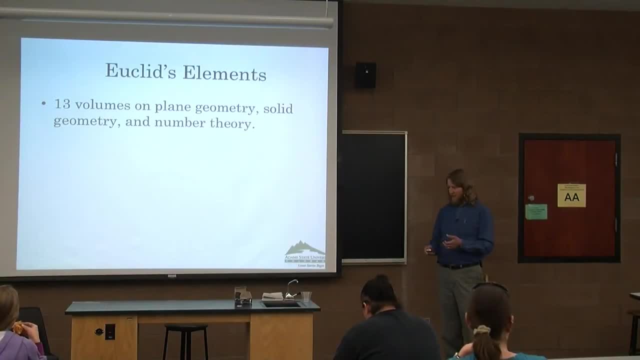 Plain geometry, solid geometry and number theory. And the peculiar thing about Euclid's Elements is that most of what he wrote was already known at the time, And so why did he get such credit for writing all of this stuff down? Well, it was the way he did it. 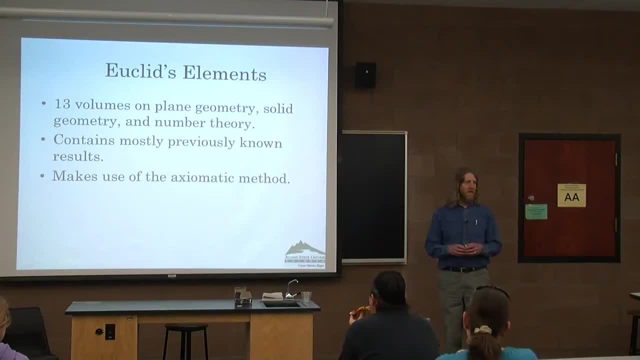 Because he made use of something that we now call the axiomatic method. I mean up to then, for instance, Thales, who was before Euclid, knew about several congruence results for triangles, For instance, that side-side-side correspondence between two triangles meant that you had congruent triangles. 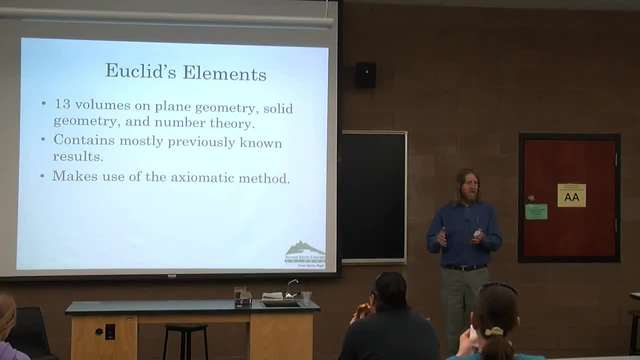 But in Thales' time, prior to Euclid, these were very much ad hoc. Hey, this works, It works great. Why does it work? It works, Why do you care? And so what Euclid did is he sat down and systematized all of the knowledge. 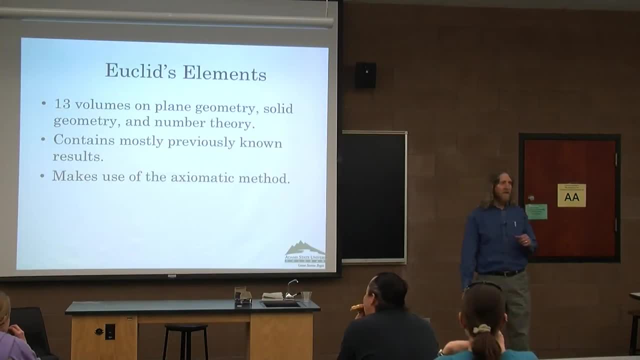 Now, of course there are some original results. I'm not going to take too much away from Euclid, But mainly the reason people paid attention to it was that it was very systematically organized around this thing called the axiomatic method. 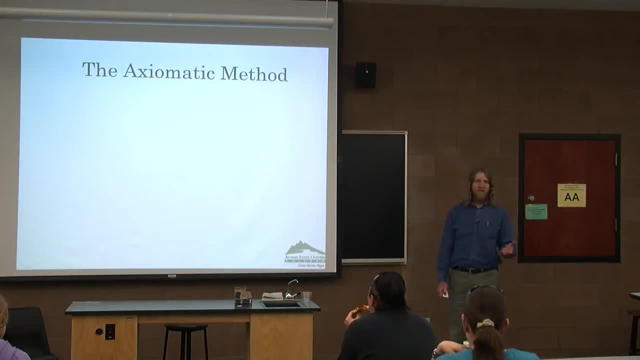 So what is the axiomatic method? Well, as the name sort of implies, you start with unproved assumptions, known as axioms or postulates. Now, it's important that these things are unproved. You don't offer any sort of proof. 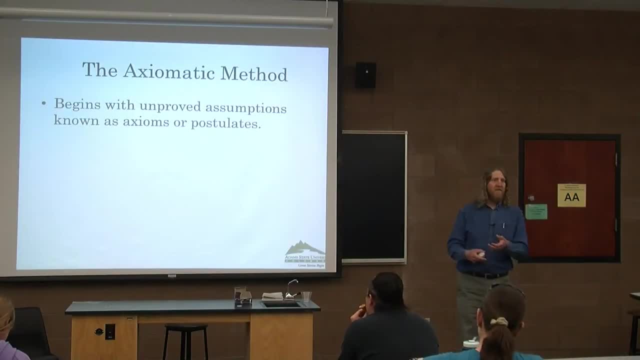 And ideally they should be obvious enough that you don't have to offer a proof. Now, obvious, I know, is a word that makes mathematicians squirm, and rightly so. So what do you do if you disagree with one of these axioms? 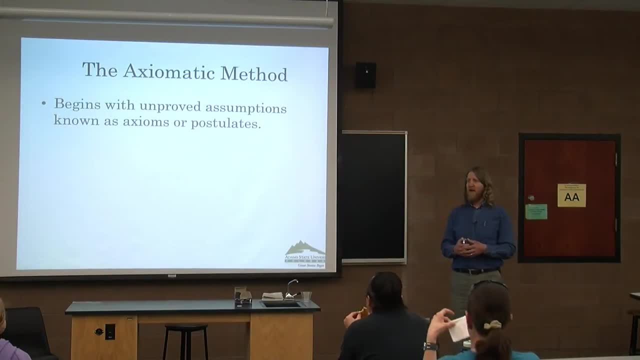 You say I don't think that ought to be an axiom. Well, it's kind of like the rules of Monopoly. I mean, what do you do if you don't agree with the rule that there ought to be $200 for passing go? 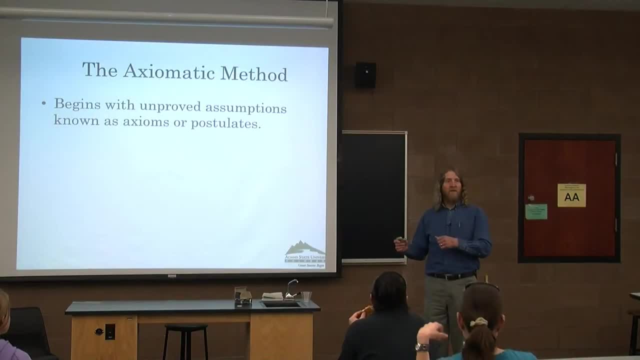 Well, then you throw that rule out right And then you play Monopoly. Now, the version of Monopoly that you're going to play is going to look very different from the version of Monopoly that somebody else plays, as far as how the game unfolds, perhaps. 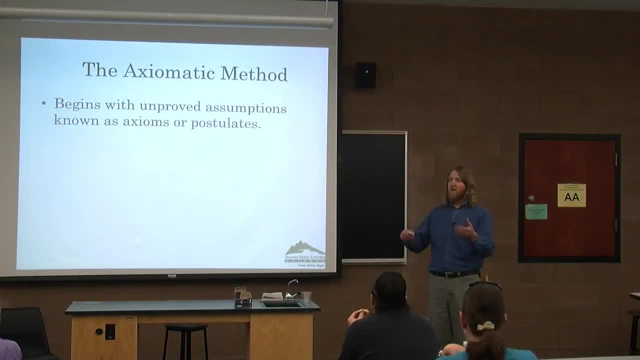 But it's still a valid game, And so if you disagree with one of the axioms, feel free to throw it out and go do your own mathematics, Use your own axioms or postulates. Then, once you set up these axioms, we all agree that we're going to have these. 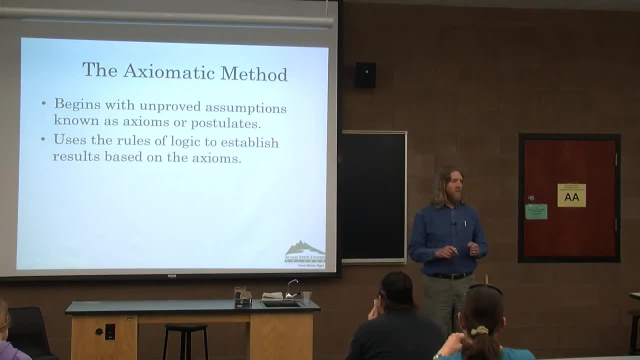 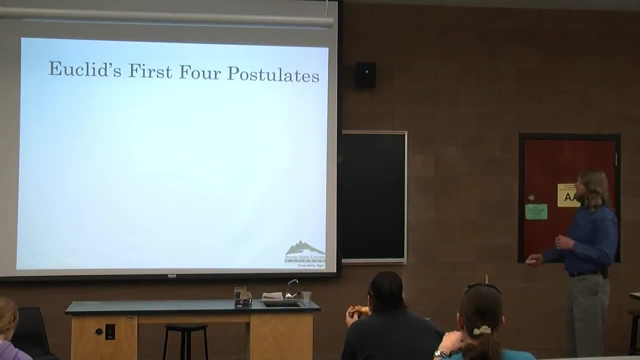 These are our postulates. Then we have the rules of logic And we use purely the rules of logic to determine further results. So let's talk about Euclid's postulates, Because he started off in his book one With five postulates about geometry. 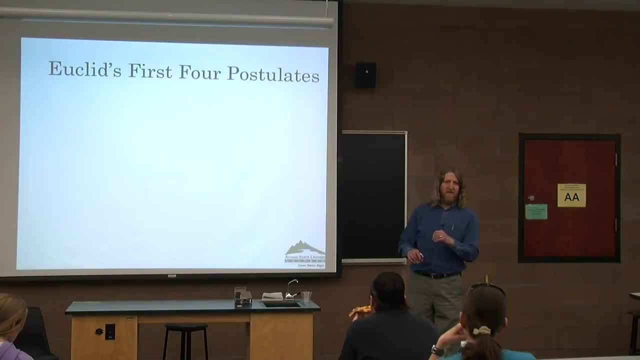 And they're worded kind of strange. I'm using the wording from Thomas Heath's 1908 translation here, And it's a little bit strange. Okay, so his first postulate says: To draw a straight line from any point to any point. 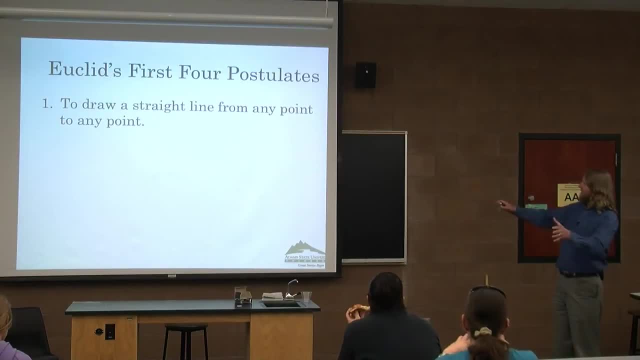 To draw. Well, it feels kind of verby, doesn't it? Well, what does he really mean? Well, in modern books you'll see this written down as Two points determine a line. Okay, so if you have two points, 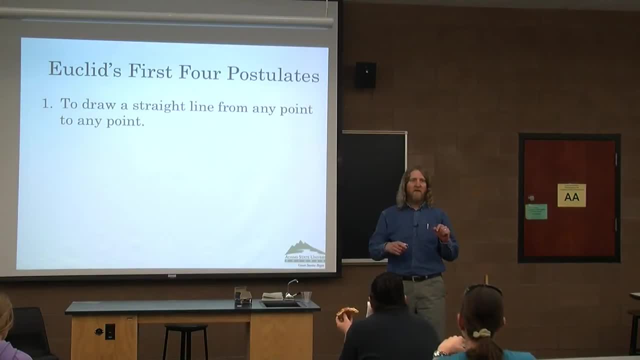 There is one and only one line that goes through those two points. That's really the modern version of this: To produce a finite straight line, continuously in a straight line. Well, what does that mean? Well, this actually shows you some of the differences in his terminology. 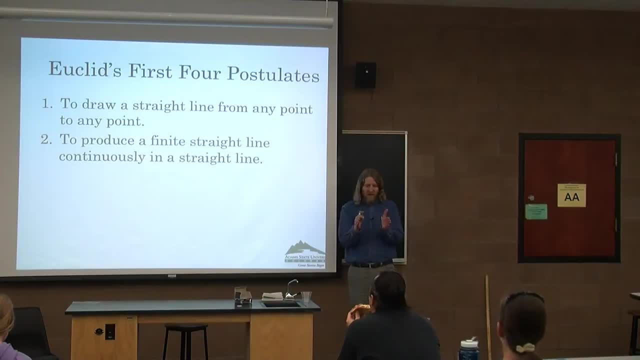 Because we wouldn't call something a finite straight line. We have another term for that: We call it a segment. So this postulate says that if you're given any segment, You can extend that segment to whatever length you like. Okay, 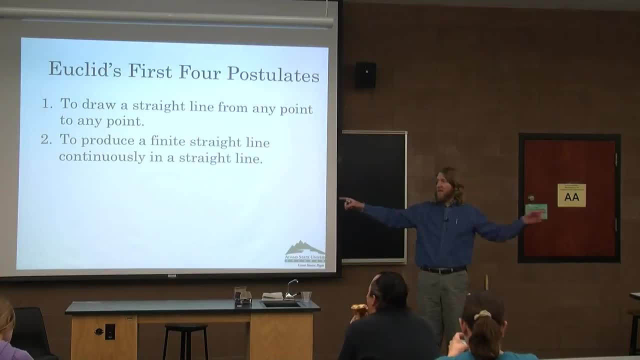 And in fact you can extend it to be an entire line, A straight line, Okay, As opposed to a finite line. So, yeah, it's a little bit weird To describe a circle with any center and distance. So in other words, if you give me a point, 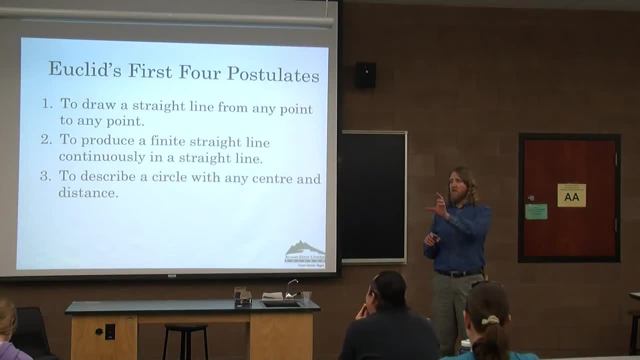 And you give me a distance, I can construct a circle around that point with the given distance as the radius of the circle. Okay, And then the fourth is that all right angles are equal to one another. Okay, And these are all fairly simple. 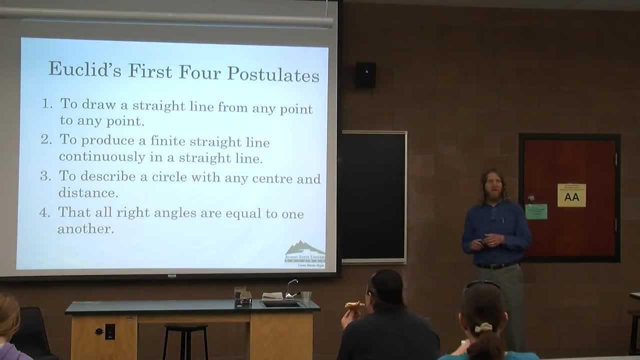 Now you may decide you don't agree with one of those And, as I said, you're free to throw that out and go do a different type of geometry, And we'll see about that in a minute. Okay, But these are the first four. 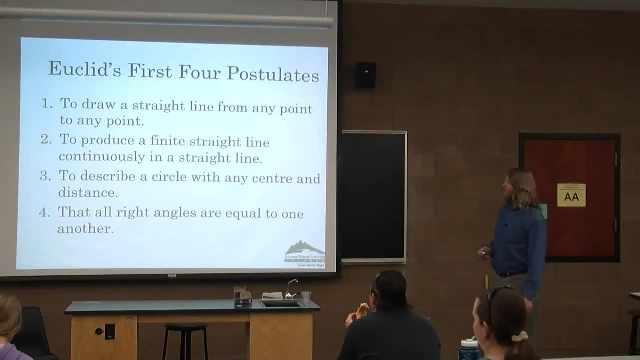 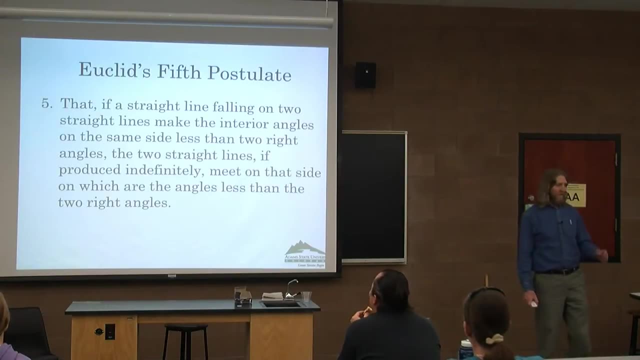 And they all seem pretty straightforward. Okay, Now contrast this with the fifth. The fifth postulate I'm not going to read out loud, I'll let you read it, Okay. So upon reading that, most people's first reaction is: 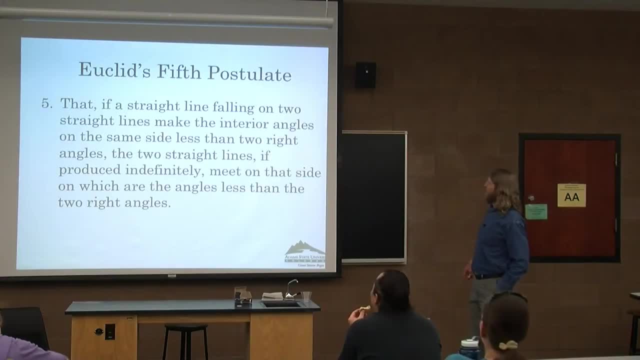 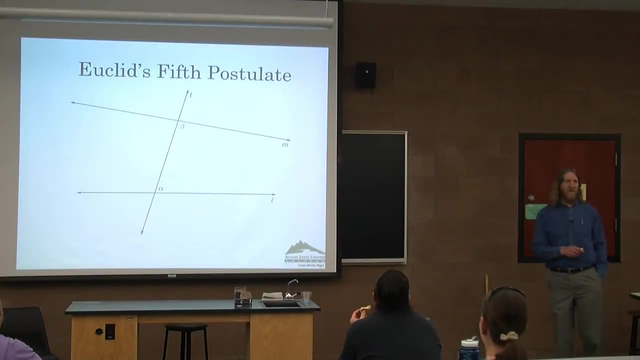 What? What the heck is he talking about here? It's certainly a little more complicated than the others. Well, I have a picture, And here's the picture, for the fifth postulate. Okay, And so what it says? So, if you have two straight lines, 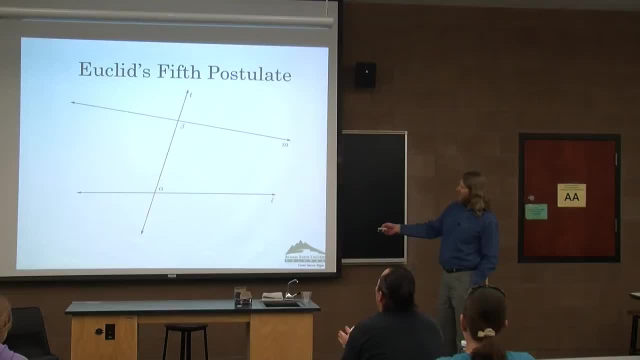 okay, which L and M here are the straight lines. and you have a third line that falls on those two straight lines in such a way that the two interior angles on the same side, in this case angles alpha and beta, those two add up. well, he says, add up to less than two right angles. 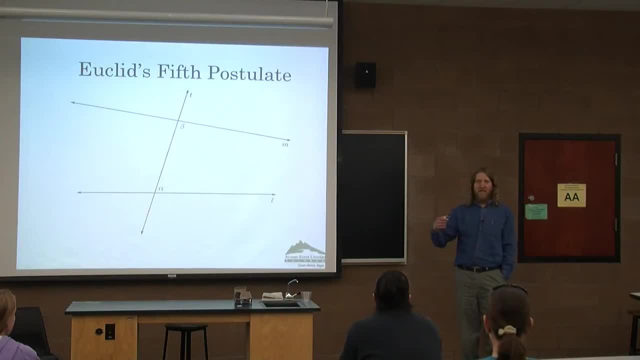 But of course we all know that a right angle has a measure of 90. And so what he's saying is: if that angle sum is less than 180,, okay, then these two lines, L and M, if produced indefinitely, will eventually meet. 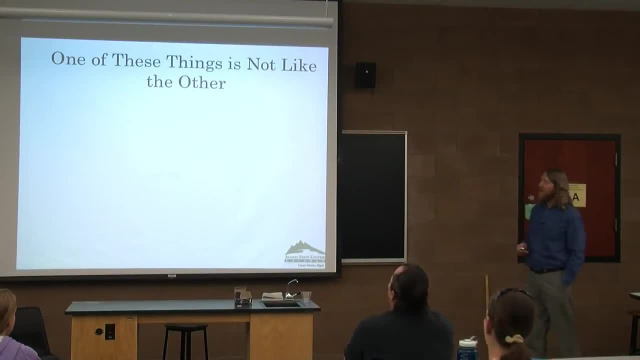 Okay, Now you might notice that of those five postulates, one of them seems a little different. right, That fifth one is quite different. First, the most obvious thing is that the first four are very short. They're easy to write down, easy to say and, yeah, that makes sense. 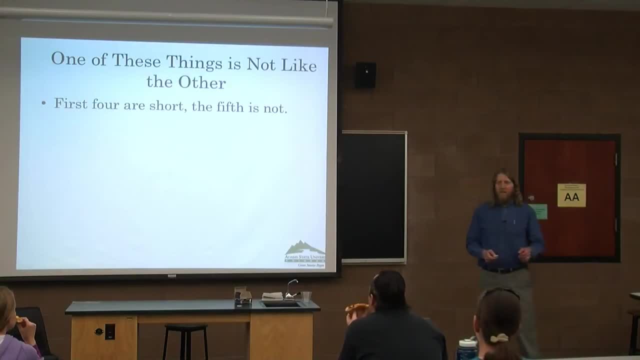 The fifth one isn't so much Okay, But the main difference, at least in my opinion, has to do with what Marvin J Greenberg calls empirical verifiability. Okay, The first four postulates are somewhat empirically verifiable. 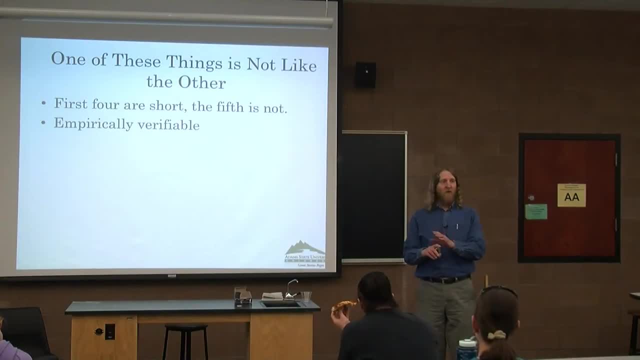 And now be careful: when I say verifiable, I don't mean provable, Because, remember, axioms and postulates are unproven assumptions that we just agree to accept, But certainly if, on the board up here, if you draw two things that represent points. 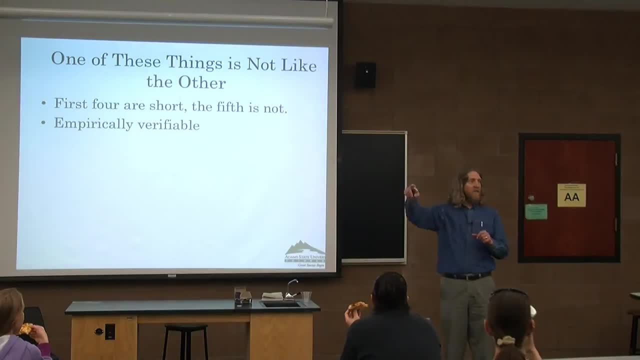 I can grab one of these meter sticks and I can make a line between them. Right, If you give me a point and a distance, I can take a compass and I can draw a circle. Okay, You say all right angles are congruent. 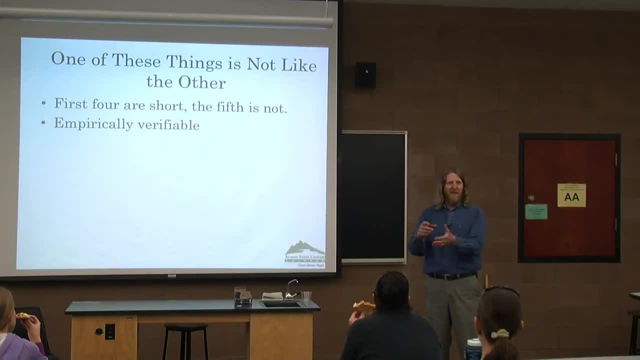 You got a right angle, I've got a right angle. We can take and compare them and see that they're congruent. So you can sort of empirically verify the first four postulates, but not so much the fifth one. And why not? 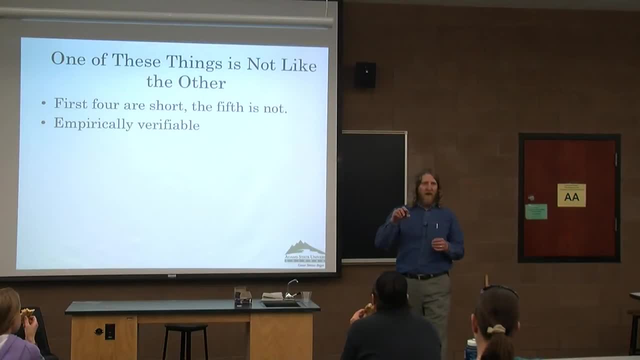 Well, the key, at least to me, is in that the term if produced indefinitely. I mean, suppose you set up a picture like I have here, All right, And you make it so that the sum of the two angles, alpha and beta, 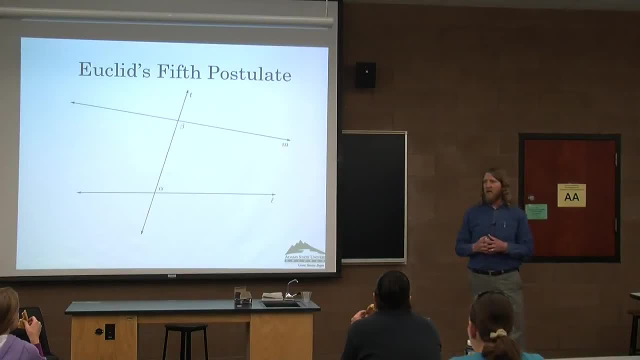 is say 179.9999999999 degrees. Okay Now, according to the fifth postulate, if I extend lines M and L long enough they should intersect, Right, But I mean, so I draw them out this far, they don't intersect. 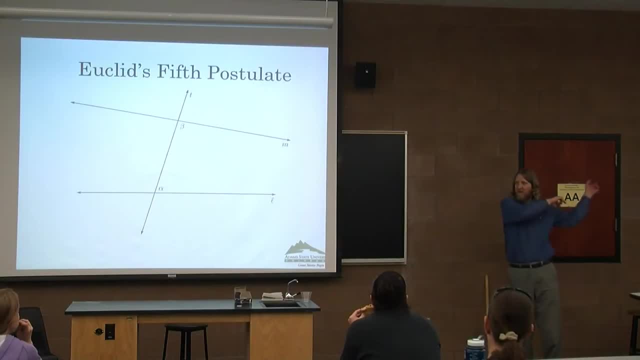 I go some more. they don't intersect. Maybe they intersect out somewhere past the orbit of Jupiter or something. It may not be physically possible for me to go out there and verify that those things intersect. Okay, And so in that sense the fifth postulate seems qualitatively different. 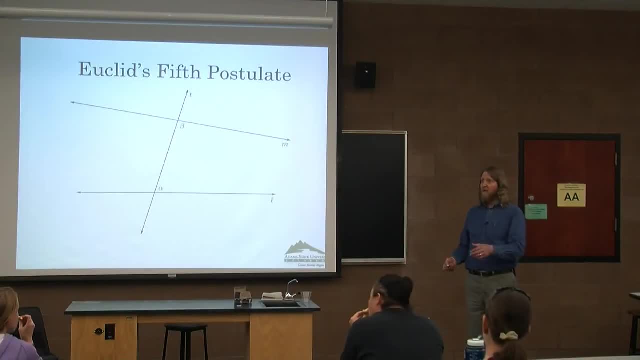 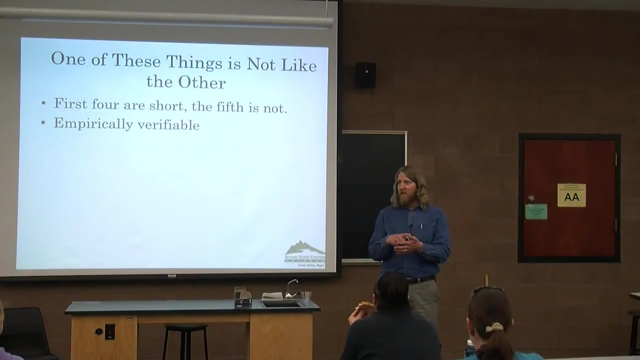 than the other four. You can't necessarily verify it. All right. So this caused problems with some early observers of Euclid Because, remember, the thing about axioms is that they're not proven. We just agree to accept them. 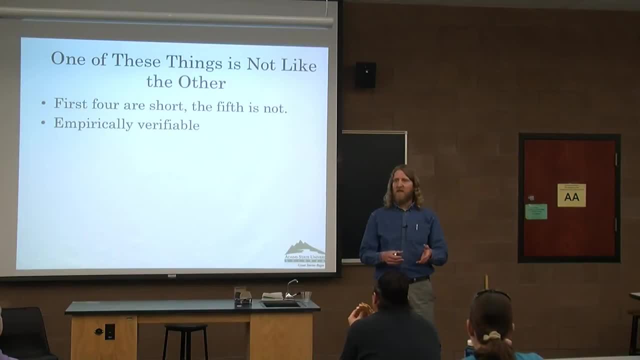 But they ought to be simple enough that we can all say, yeah, that seems to make sense. But some early observers of Euclid said: wait a minute, that one, we're not too comfortable with that, Wouldn't it be nice? early commentators thought. 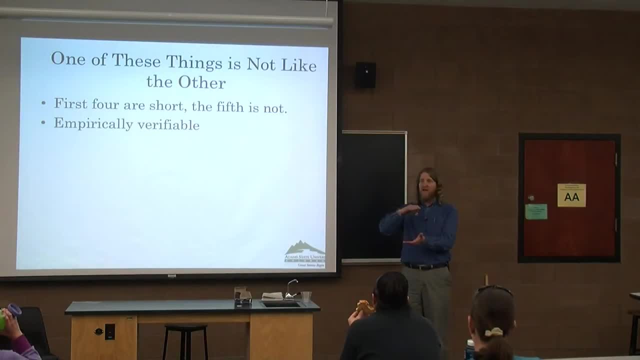 if, instead of having that fifth postulate as a postulate, wouldn't it be nice if we could prove that from the other four? Then we could clean up our axiomatic system, We could throw out this ugly-looking postulate. just keep the nice four clean ones. 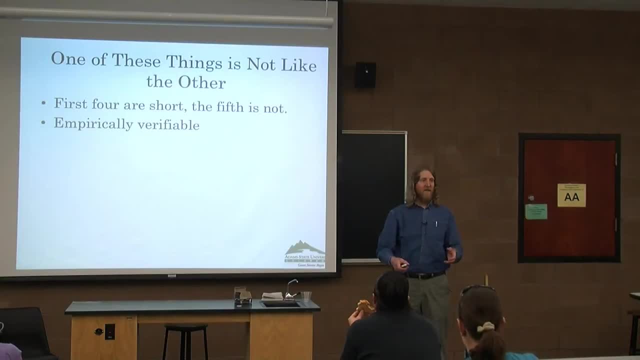 We could prove the fifth postulate as a theorem, and that would make the system a whole lot better. Okay, There are suggestions, and again, this is from Greenberg's book. there are those who claim that even Euclid himself was squeamish about this. 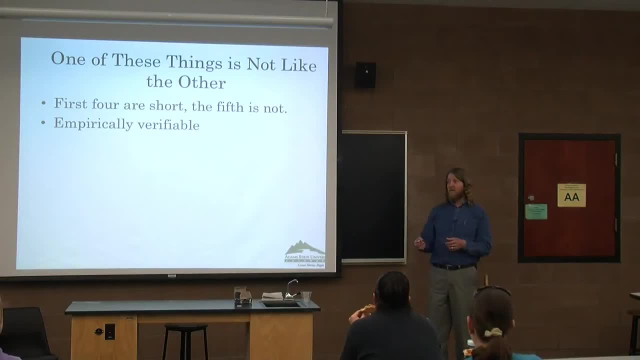 but the only evidence that they offer to me seems to be that he waited until he waited as long as possible before he started using the fifth postulate. So if you read his Elements, Book 1, he has the postulates. he starts proving theorems. 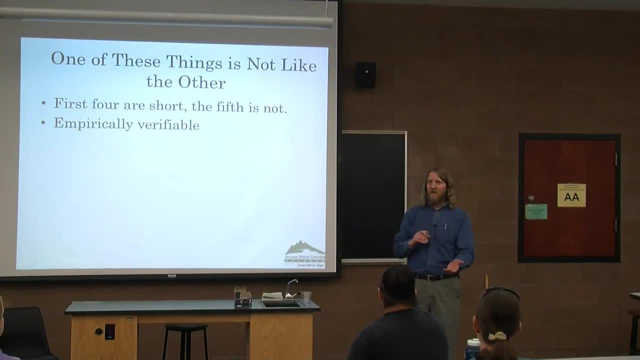 and so he has. I think it's the 29th theorem, before he actually ever uses the fifth postulate for the first time And, as I say, many commentators suggest that that means that Euclid himself was a little squeamish about the fifth postulate. 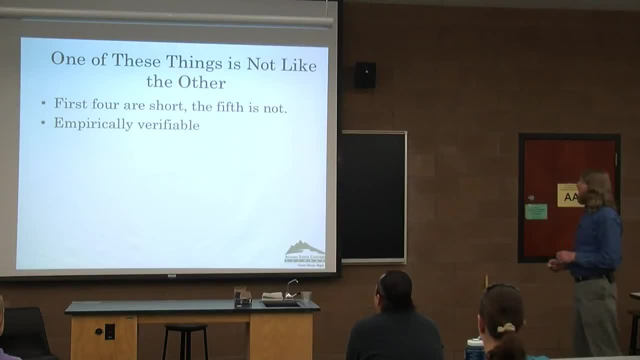 I'm not sure I buy that line of reasoning too much, But one of the earliest commentators on Euclid was a guy named Proclus, who lived well 700 and some years later. Okay, Proclus is rather famous as an expositor and a critic. 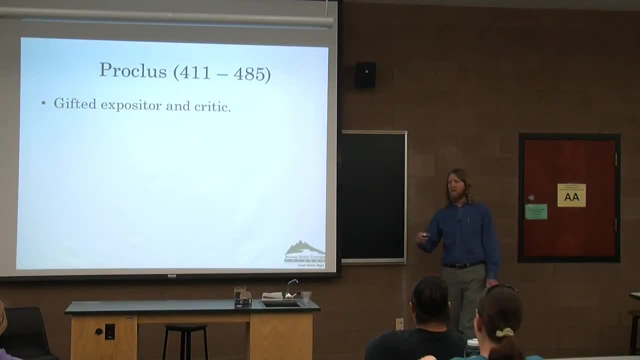 He never actually created any original math of his own, but he wrote extensively on other people's works And of course he wrote- well, as I say, wrote- introductions and commentaries for many other works And he wrote a commentary on Euclid. 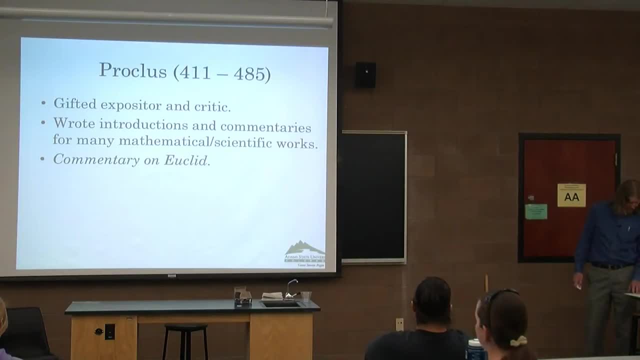 And in his commentary on Euclid, he gave what is the first recorded attempt to prove Euclid's fifth postulate from the other four. Okay, And I'll try to give you an idea of how he did it. Okay, So his proof, which, you'll notice, is in quotation marks. 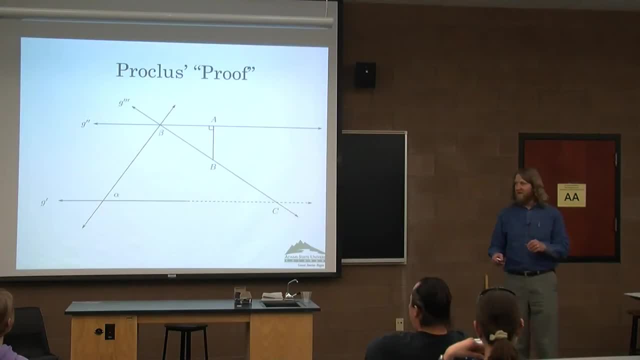 works something like this. This is a very complicated picture, so let's talk about what's going on. So he starts with a line G prime. Is that visible? Okay, He starts with a line G prime and then he does something a little squirrely. 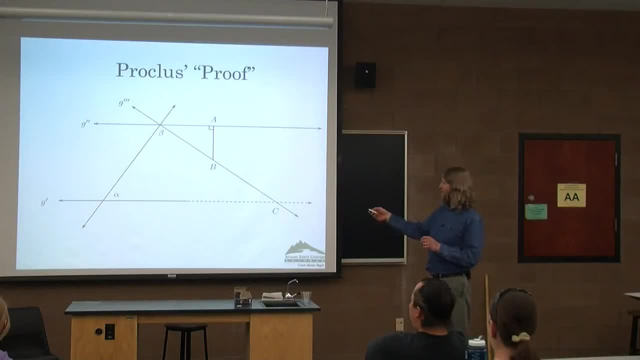 He constructs a line G double prime. Gotta love modern notation as opposed to this. That's parallel to the line down here. Wait a minute, that's a problem, But not too big a problem. Then he says: alright, now let's make this third line. 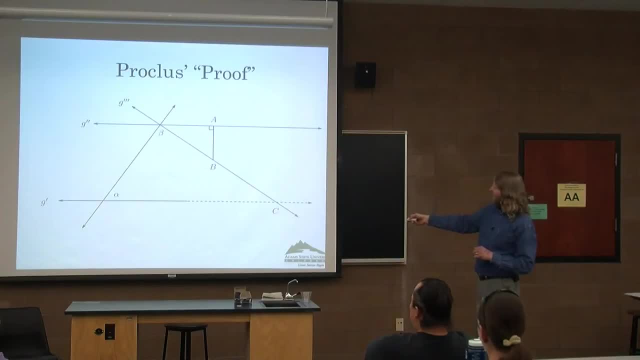 G triple prime. okay, so that we have two angles, alpha and beta- here that sum to less than two right angles. Okay, so alpha plus beta is less than 180 degrees. And what he does is he comes out and he picks a point B. 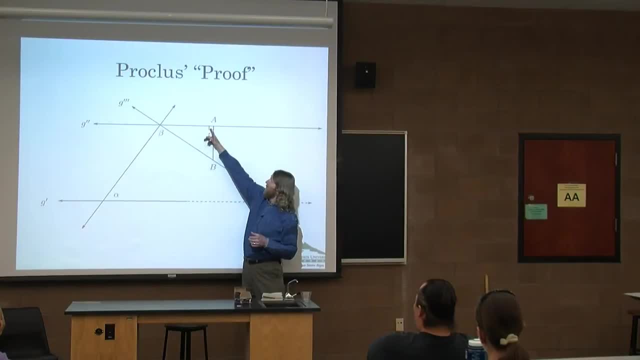 and he erects a perpendicular from this point to the line G. double prime at this. point A: Okay. He then proceeds to argue that the distance AB gets larger the farther down here you move. point B: Okay. And so at some point the distance AB. 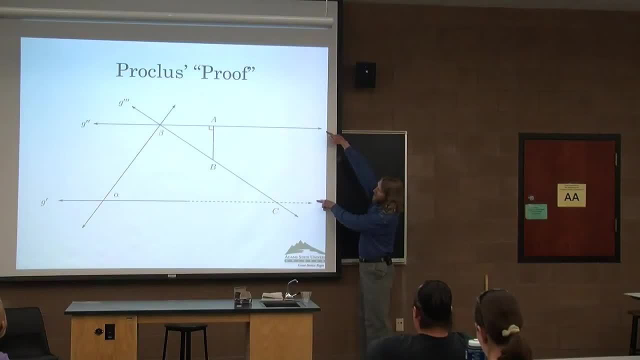 must exceed the distance between the two lines G prime and G double prime. Okay, And therefore the lines will then be intersecting, Okay. So again to recap, he says: this distance grows as you move point B out here, And eventually this distance will exceed. 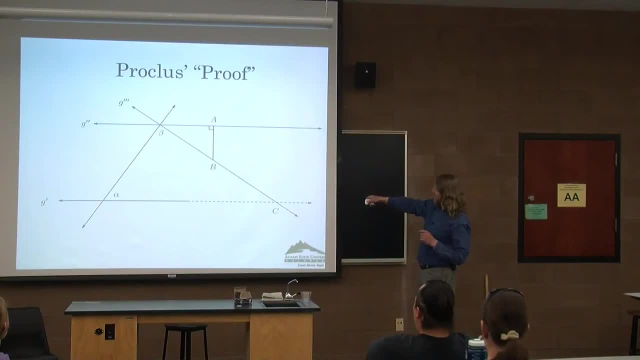 the distance between these two lines, and so when it first matches that distance, in fact you're going to get a point of intersection between the two. All right, Now, that was wrong. It was wrong for a variety of reasons, but the most egregious problem is: 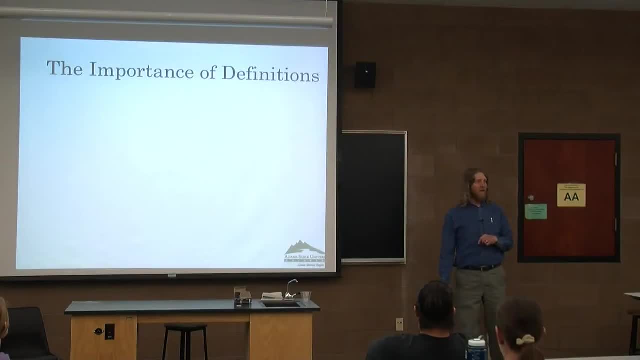 well, what does it mean for two lines to be parallel? It simply means, well, that they lie in the same plane and they do not meet. Okay, But Proclus tacitly assumed that parallel lines are everywhere equidistant. And that's kind of consistent with your experience. 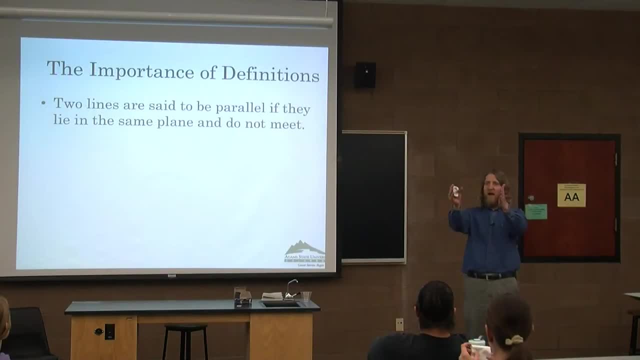 When you think about parallel lines, most people you visualize like railroad tracks. Right, They're the exact same distance all the way apart. But there's nothing in the definition of parallel that says that. It simply says they do not meet. Okay. 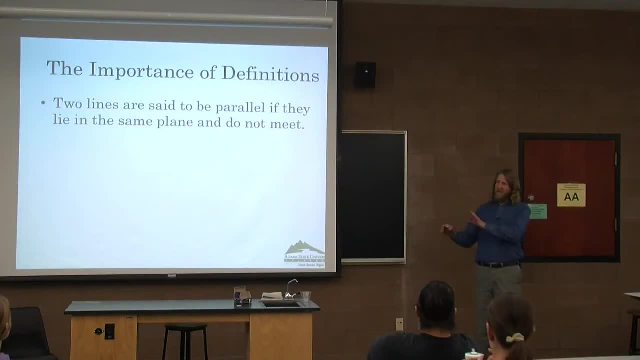 He also used a parallel line in his construction which isn't supported by the other postulates, and that's a problem too, But the main problem is that there's nothing in the definition of parallel that says anything about equidistance. Okay, 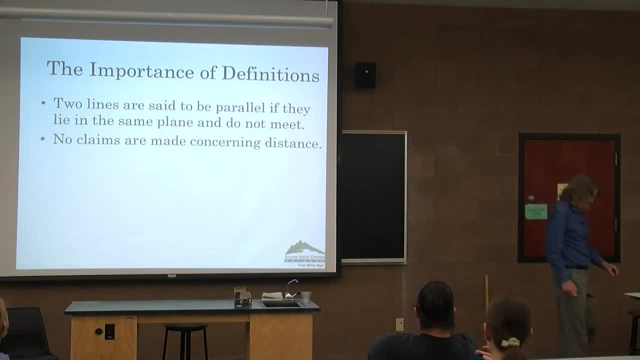 Hmm, So now, while we're on the topic of definitions, I want to talk. it's important. definitions are important, but they're also kind of dangerous. Okay, And modern mathematicians have accepted the fact that there are some terms you cannot give. 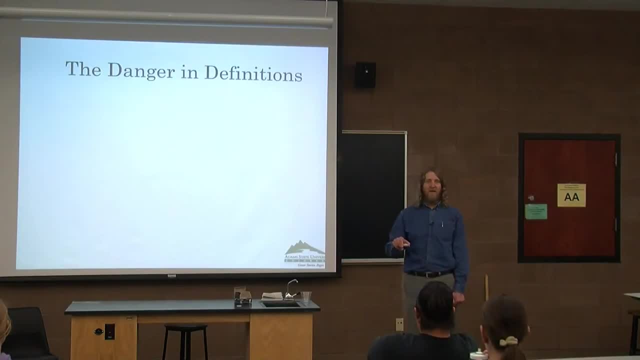 a rigorous definition for, In fact, in geometry, point line plane, those are terms that we don't try to define. Wait a minute. What do you mean? you don't try to define them. Well, I mean, how could you? 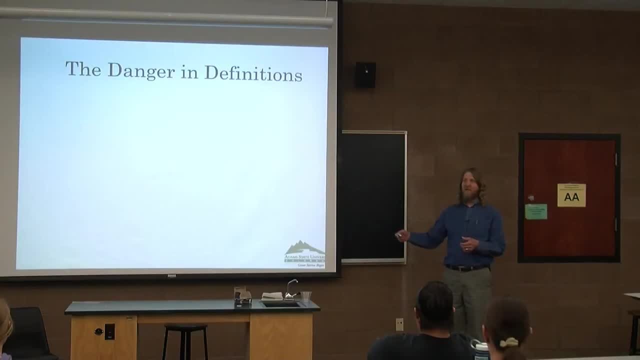 I mean, even Aristotle realized, even before the time of Euclid, that rigorous definitions are ultimately going to be circular. Okay, If you don't believe it, try an experiment. Look up a word like noise in the dictionary and then you see it says sound. 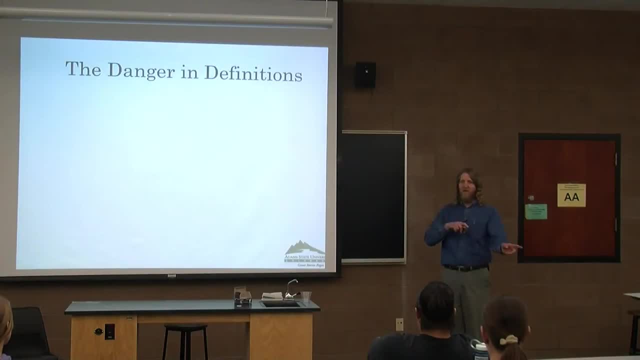 and you look that word up, and then you look a word and pretty soon you're back to the word noise. I mean, you've just gone in a big circle. And so now Euclid, he did, He tried, He gave definitions for all of these things. 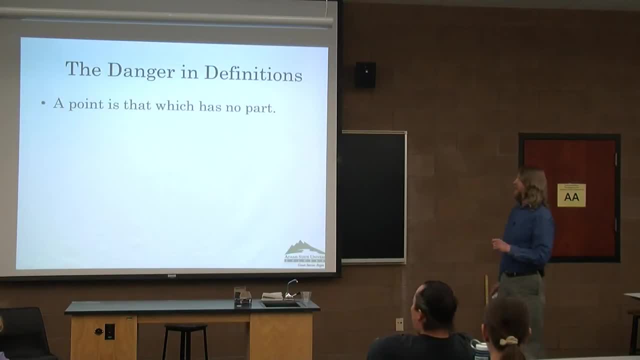 and he defined a point. And what did he define it? as That which has no part. So a point is nothing, then It's got no part. A line- Here's a good one- A breadthless length. What does that mean? 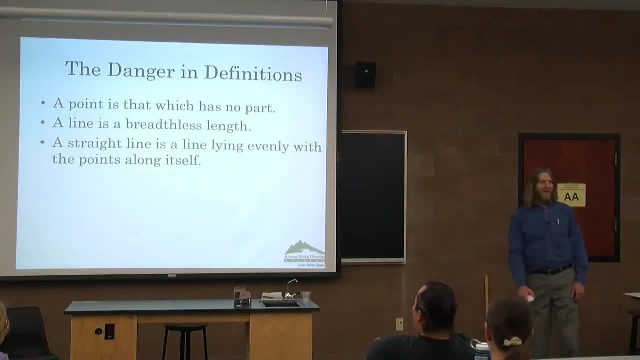 And my favorite, a line lying evenly with the points along itself. What, Okay? So in modern geometry we just accept that things like point, line and plane are undefined terms, And so Hilbert gave a famous example that all of the theorems ought to be true. 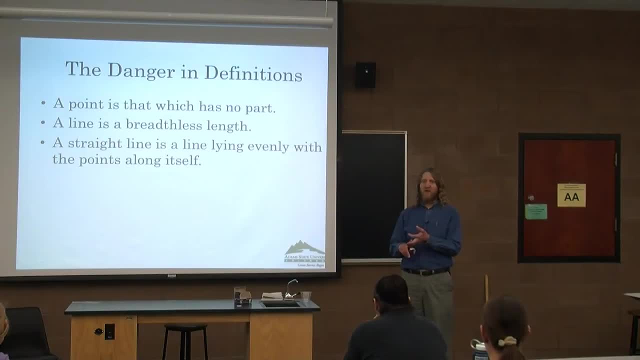 if you replace those terms by other terms. So, for instance, if you replace your postulate about two points determine a line- and I think his example was, you know, two beer mugs determine a table, then all of the theorems ought to still be true. 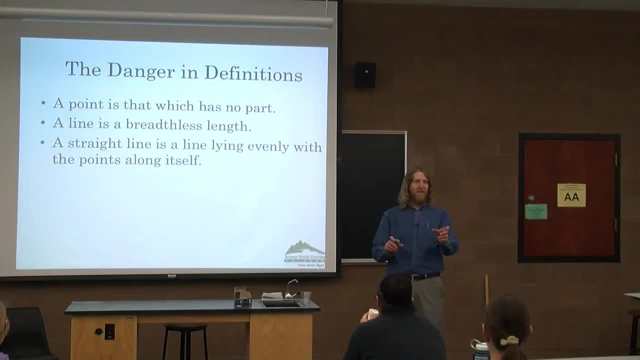 with point replaced by beer mug and line replaced by table. Or you could do something even a little more generic. You could say: two alphas determine a beta- Okay, And then you could prove theorems about alphas and betas, And it doesn't matter what a point and a line is. 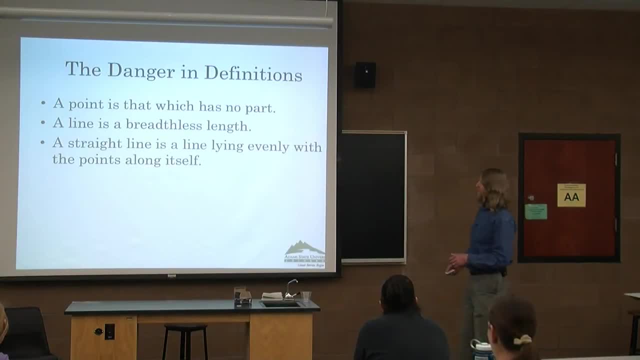 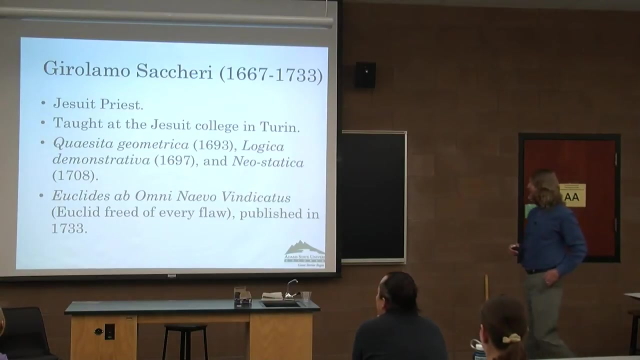 Okay, The theorems should still be true. All right, Okay, So yeah, We accept the need now for undefined terms. Oops, Wait a minute. Hmm, Okay, Those were supposed to come in one at a time. The next notable. 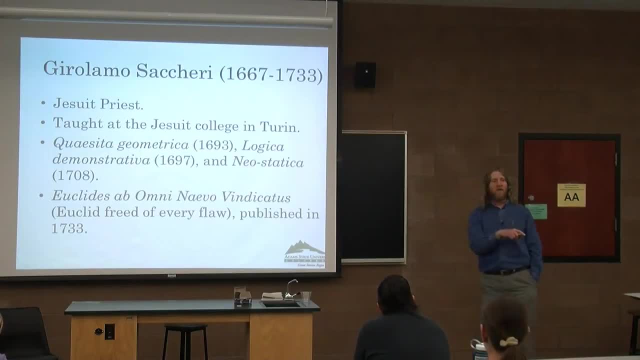 the next notable attempt to prove Euclid's fifth postulate is by a Jesuit priest named Sicarii Okay. He taught at a Jesuit college in Turin and you see he had some experience with mathematics. He wrote several books. 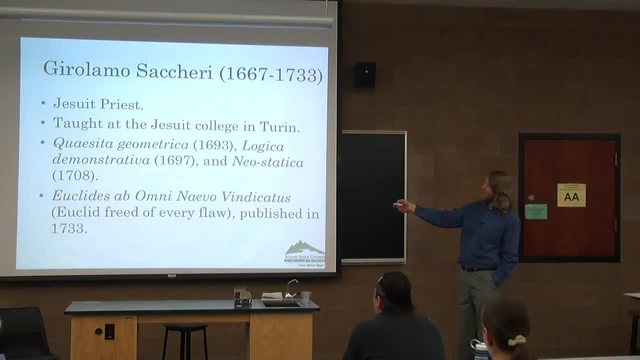 This one is several little pieces of geometry, I think is sort of roughly what that? but a book on geometry, a book on demonstrations in logic, a book on statics. So he kind of knew what he was talking about. At least he was a well-educated. 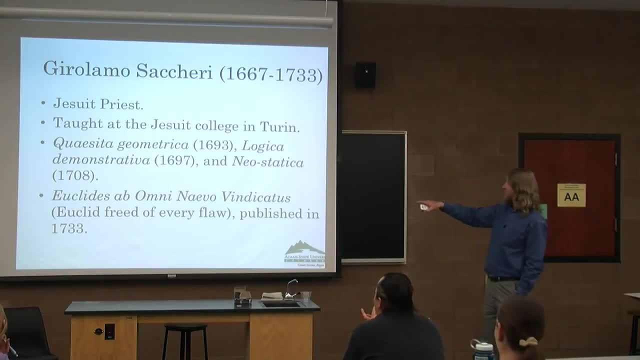 well-educated fellow, And in 1733, just before his death, he published this one, which that's the Latin version: Euclid freed of every flaw. Okay, Euclid freed of every flaw, And in it he proved Euclid's fifth postulate. 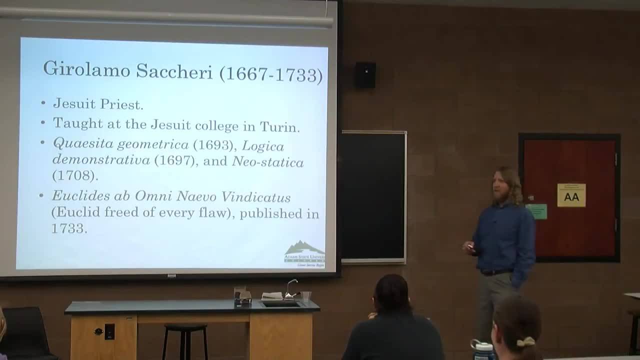 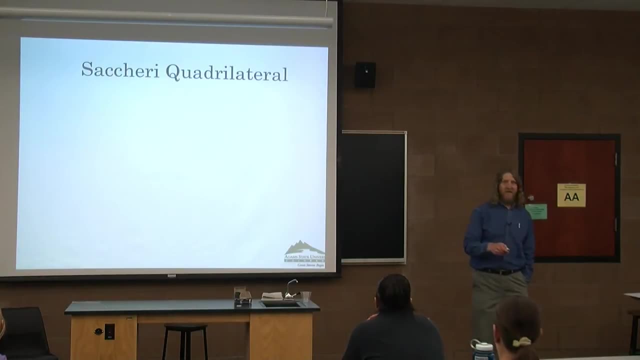 from the other four At least. he thought he did Okay, And here's how he did it: Okay, He constructed a thing that has become known as the Sicarii quadrilateral. Okay, And the Sicarii quadrilateral is constructed. 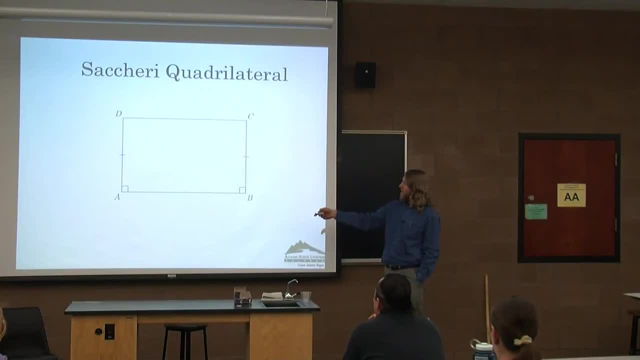 You start with a segment that we'll call AB. Then you erect two perpendiculars- all right- that are the same length. All right, That's what this means. This is the congruence symbol from geometry. Okay, So you erect two perpendiculars. 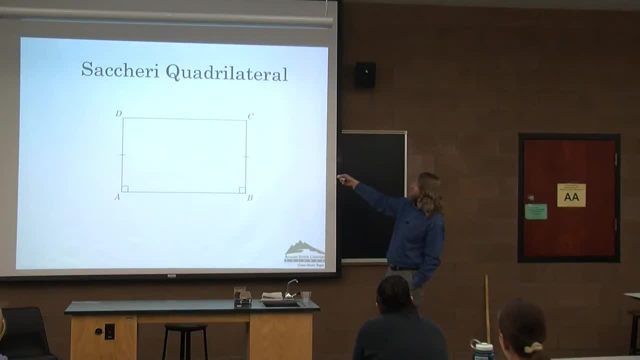 that are the same length, and then you attach the two points together at the top Right, Which we can do because two points determine a line. All right, And he rightly figured that if he could prove that these angles at D and C were right angles. 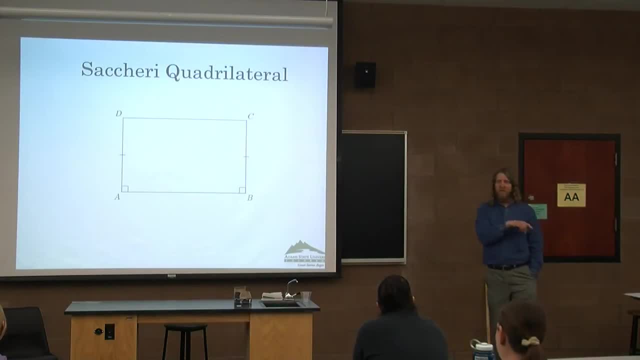 okay, then he would have proved Euclid's fifth postulate- Okay, In a way that I can make precise later if you're interested. Okay, Well, it wasn't hard for him to show that the summit angles here, that's what we'll call these. 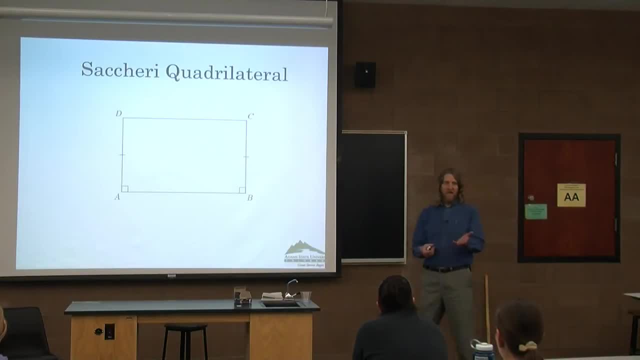 that the summit angles must be congruent. Okay, That's actually a fairly easy proof, Doesn't require anything. with the fifth postulate, Just with the first four, you can prove that the summit angles must be congruent. So then you wind up with three cases. 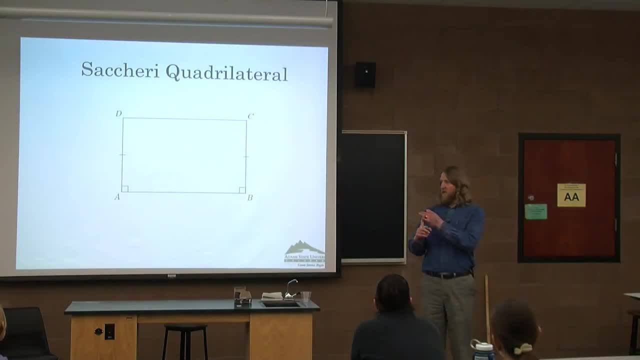 Either both of the summit angles are obtuse angles, or they're both right angles, or they are both acute angles. Okay, He was able to dispense with the hypothesis of the obtuse angle. He showed that they couldn't possibly be obtuse. 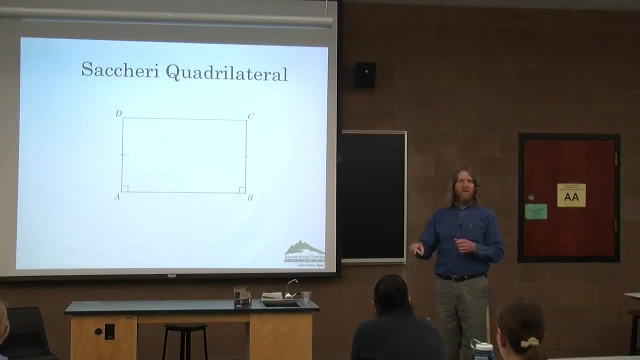 But, try as he might, he could not prove that. the angles could not be obtuse, They couldn't be acute, And he tried for quite a long time. As you noticed, this was published just before his death. He'd been working on this for a very long time. 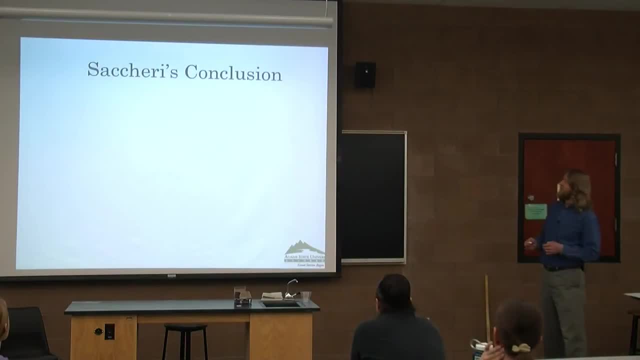 And he finally decided that he had done it Okay, And he proved that Euclid's fifth must be true, because to think otherwise is repugnant to the nature of a straight line. Repugnant to the nature. So proof by disgust. 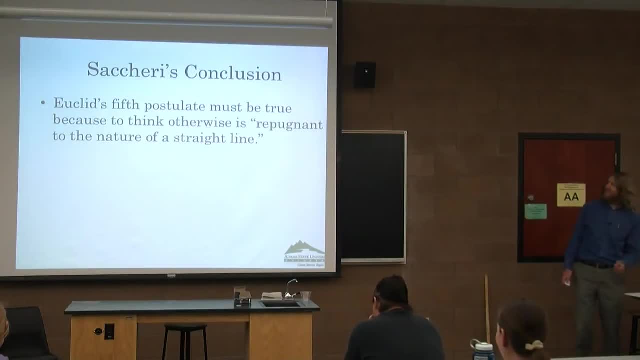 I guess, is the term there. Now, these are just two of the failed attempts. There were many more. How many? Well enough that in 1763, a mathematician named GS Kugel wrote his doctoral thesis on failed attempts to prove. 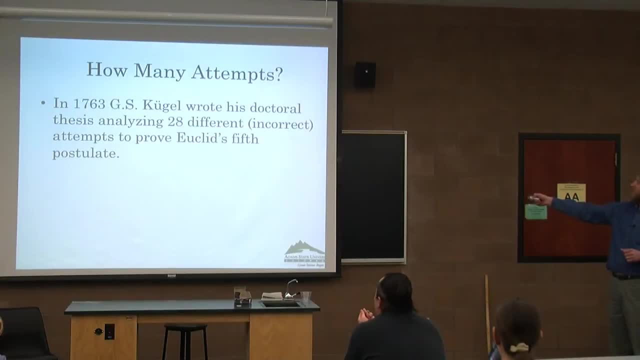 Euclid's fifth postulate And it analyzed 28 different attempts- failed attempts- to prove Euclid's fifth postulate. So I mean it was a bit of a cottage industry for a long time trying to prove Euclid's fifth postulate. 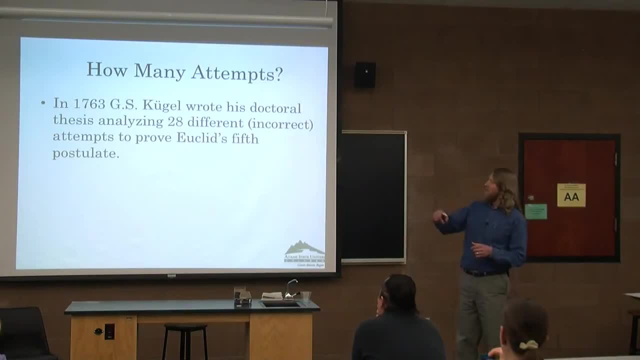 from the other four. Well, what I've showed you thus far were two direct, two attempts to prove Euclid's fifth postulate by direct proof. But, as my Math 250 students know, there are other techniques. Like what Math 250 students 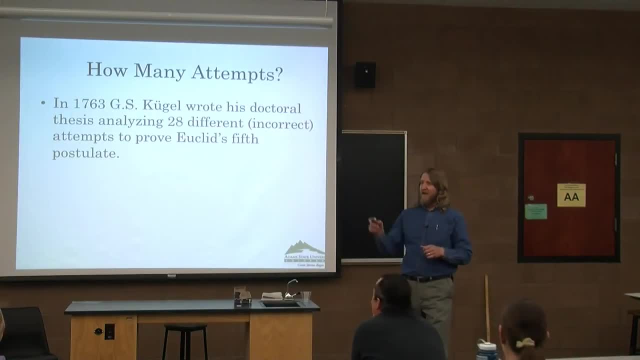 What's another technique other than direct proof? And Or Keep going The big one Contradiction, Proof by contradiction. In a proof by contradiction, what you do is you assume that the result that you're trying to prove is false. 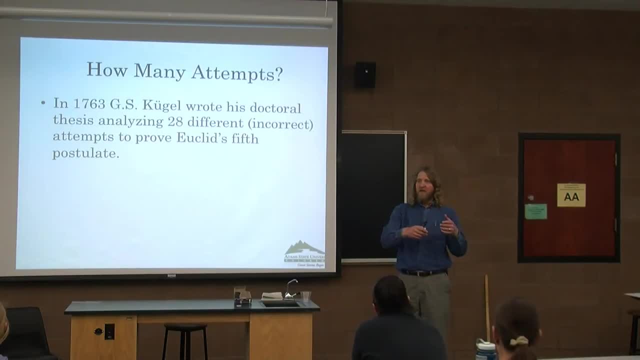 And then you try to derive some sort of contradiction, So you assume that the thing is false, and then you are able to prove that one equals two. Well, if you can come to a contradiction like that, then provided all of the steps of your logic, 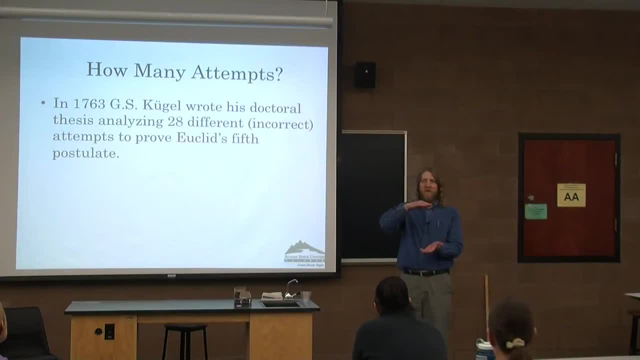 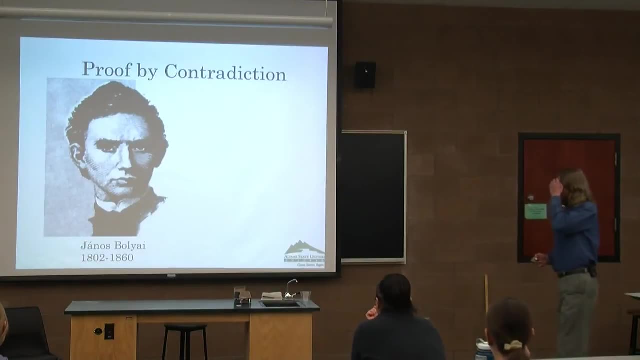 were correct. something's got to be wrong, And the only thing that could be wrong is your assumption that it was false. Therefore, it must be true, Okay. Well, so a young Hungarian mathematician named Janusz Bolyai used proof by contradiction. 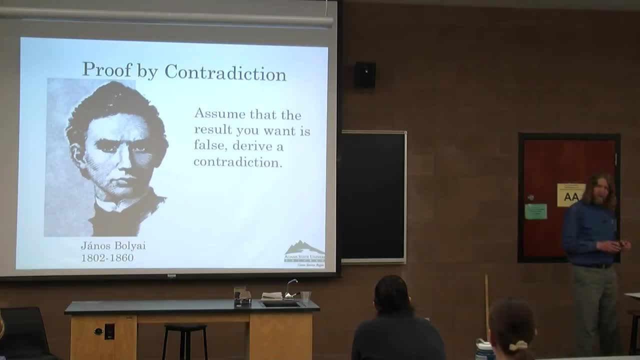 to attempt to prove the to prove Euclid's fifth postulate from the other four. Alright, Well, so that means that you have to write down the negation of Euclid's fifth postulate. Okay, so you have to come up with a statement. 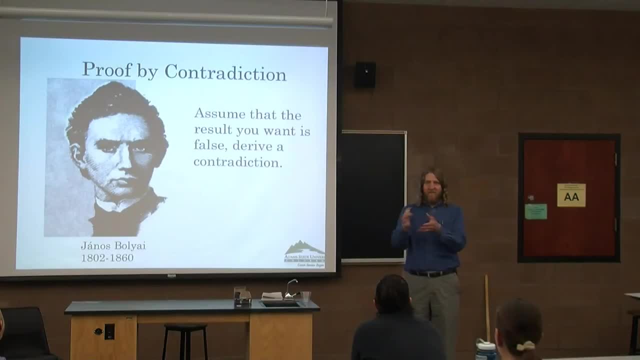 that is logically equivalent to the negation right, the. not that Well, if you go back to that slide, which I won't, but if you look at the way Euclid's fifth postulate was written, it's a nightmare to try to negate that. 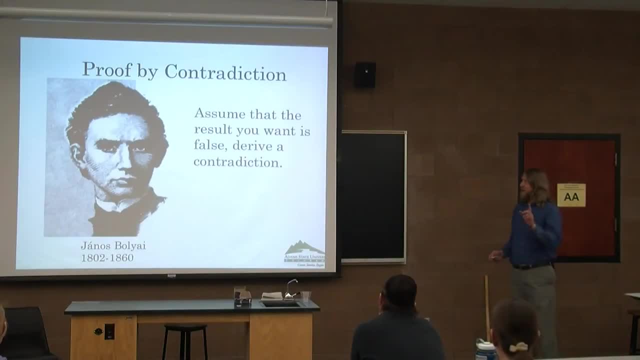 So what we actually usually do is we negate an equivalent form. Okay, And the equivalent form of Euclid's fifth postulate was the one I'm going to use. was developed by a mathematician named John Playfair, which isn't that a great name. 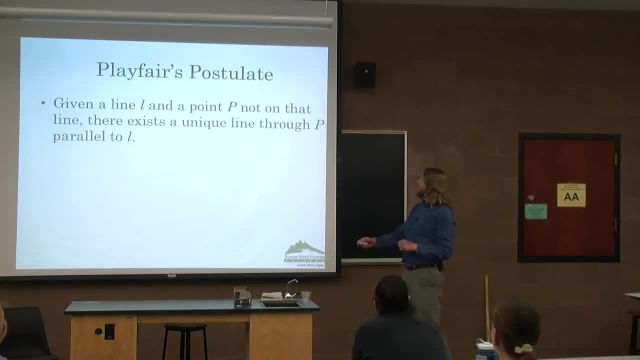 Playfair, Playfair, you. Okay, Anyway, And this is what he came up with, And this is the statement that you find in most modern geometry texts, like in high school geometry texts: Given a line and a point, not on the line. 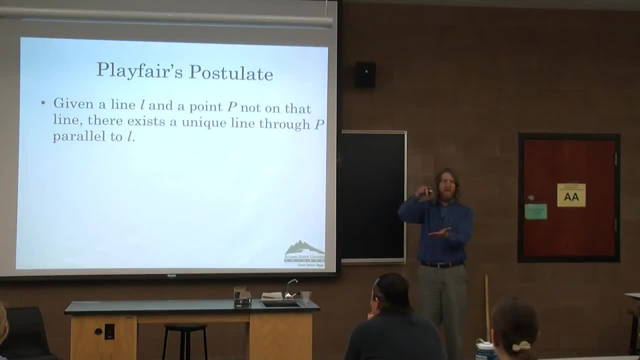 there is exactly one line through the point parallel to the given line. Okay, That's Playfair's postulate, And it turns out that you can show that this is logically equivalent to Euclid's fifth postulate. Right, And so Bolyai decided to negate this. 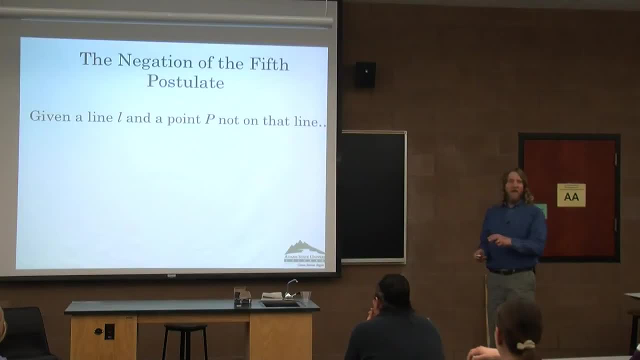 Okay, Well, there are two ways that you can negate it. All right, So you start off. you got your line L and your point P not on the line. There are two ways to negate the postulate. One is that there are. 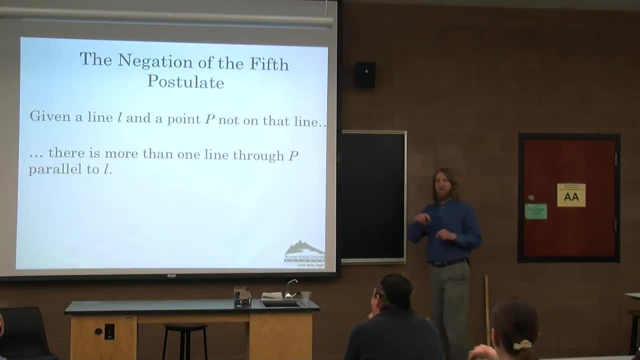 there's more than one line through P. Right, Because remember, Playfair says there's exactly one. So you can negate it one of two ways: You can either say there's more than one or that there are no lines through P. 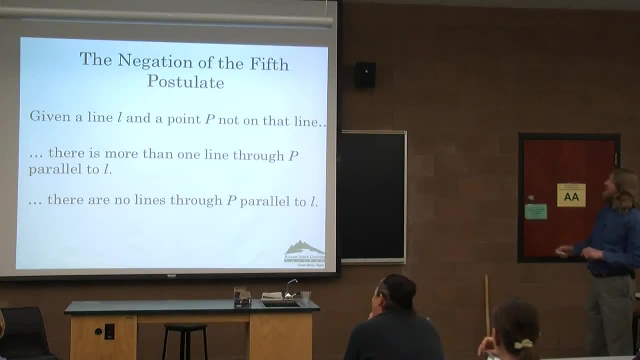 parallel to there, to the given line Okay, And using this, set up the Bolyai attempted to find contradictions, some sort of contradiction somewhere, based on these negations, And this slide shows you a complete list of all the contradictions he obtained. 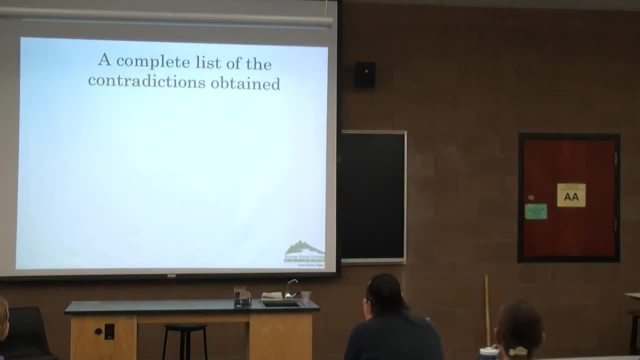 And that's it. He didn't find any contradictions. Now, to be sure, he found theorems that were bizarre. Okay, He found results that did not agree with the normal geometry, most notably the angle sum of a triangle, which we're going to talk about in depth. 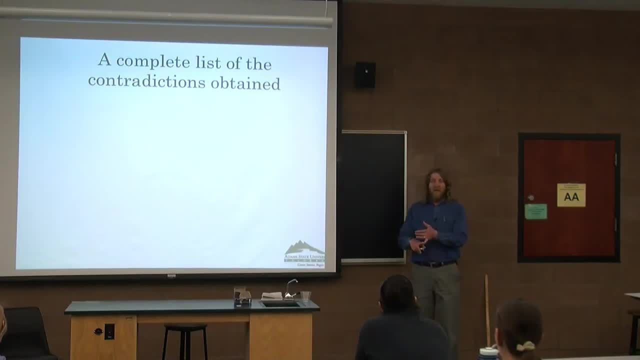 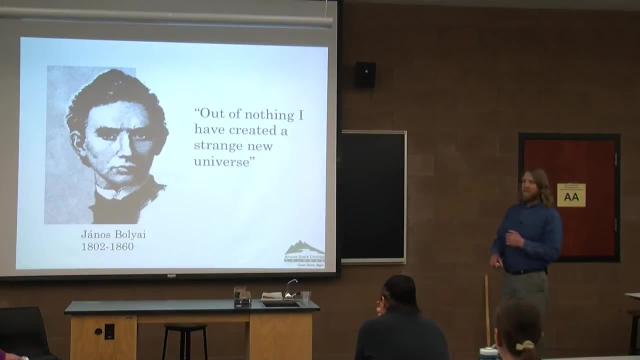 here in a few minutes, Okay. But he didn't get any kind of contradiction, And so this led him to say in 1829, out of nothing I have created a strange new universe, So somewhat bold Well. 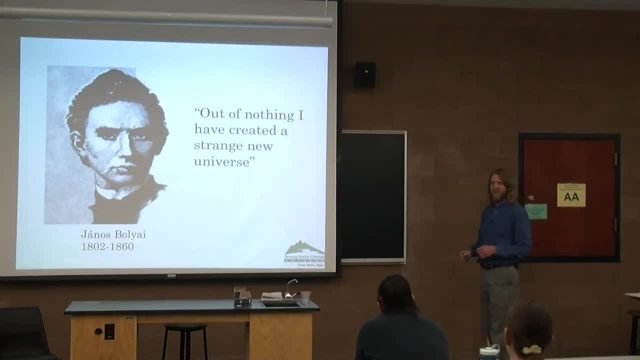 now a little bit of lesson about Bolyai. Bolyai- well, actually, at this point, Bolyai, he was the first person to have ever been, to have ever been, to have ever been, to have been, to have ever been. 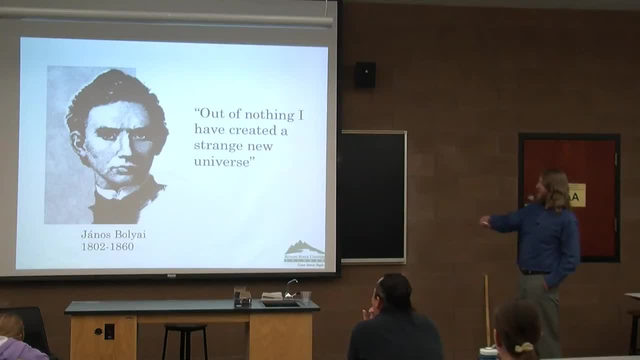 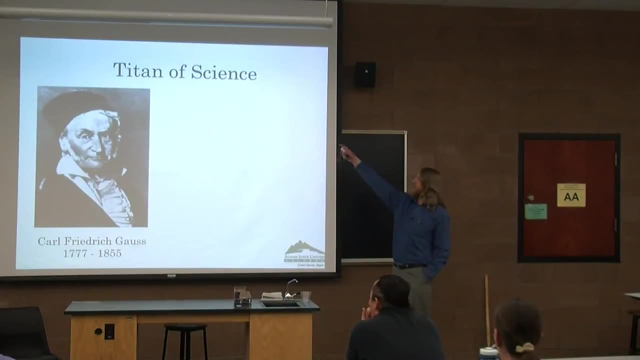 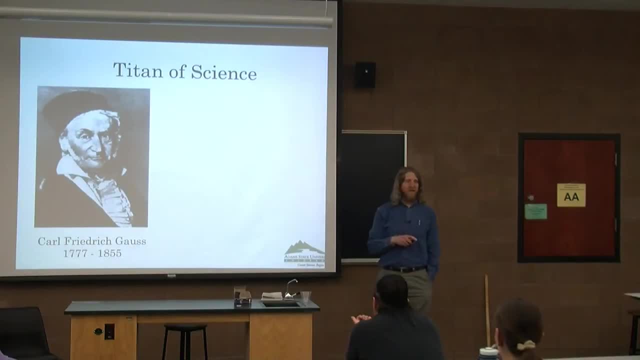 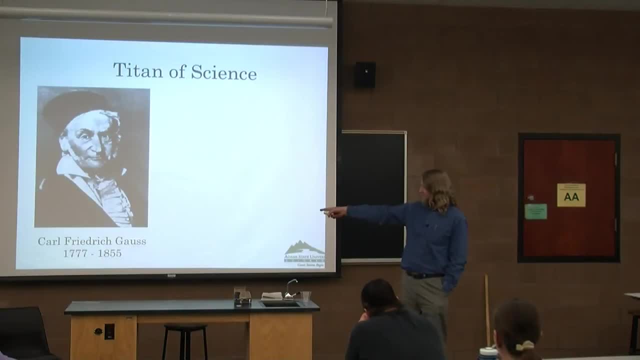 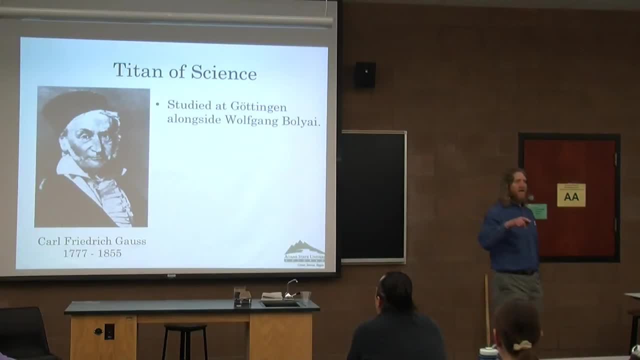 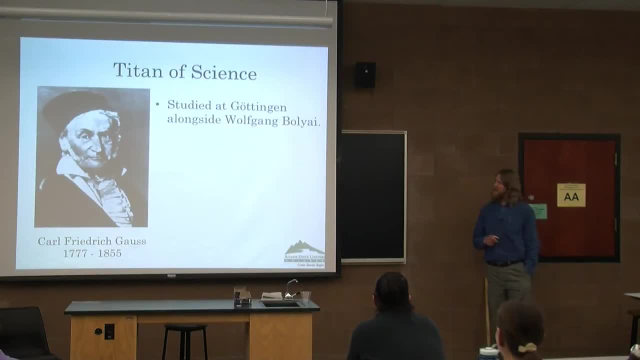 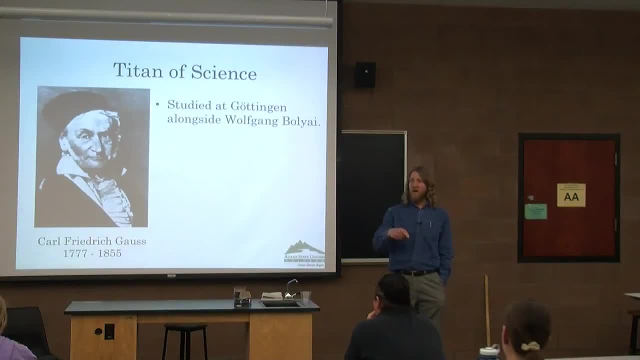 early age and had already contacted Gauss and tried to get Gauss to take him in as a pupil or an apprentice and Gauss had already refused. You know, I'm really I'm too busy to take a little kid here. I don't care how smart. 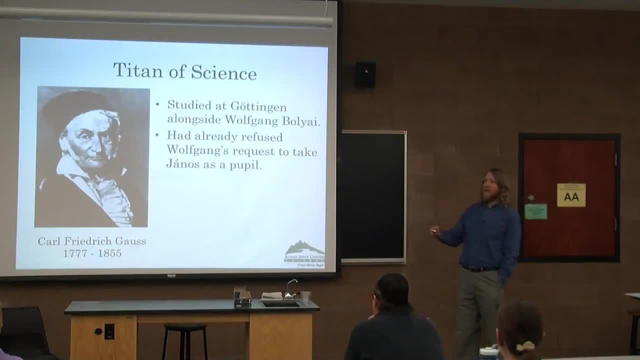 he is, so he'd already turned that down. Well, when Bolyai the younger came up with these results, this strange new universe, his dad was excited. oh wait. so he sent these results off to Gauss and said: hey, 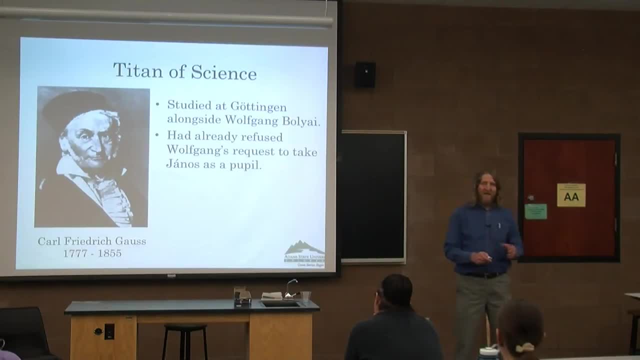 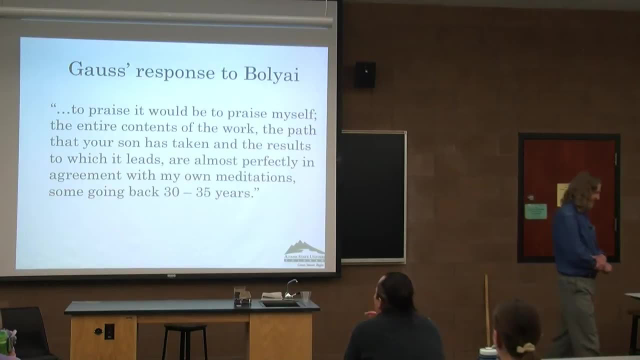 you're going to love this. my kid came up with this. tell me what you think. Gauss got them and read them and here's his response. he says: I dare not praise it too highly because- yeah, because- the entire contents of the work. are almost perfect. I was perfectly in agreement with my own meditations going back thirty to thirty-five years. So, yeah, the original hipster right. yeah, I knew that before. it was cool, I did that thirty years ago okay. 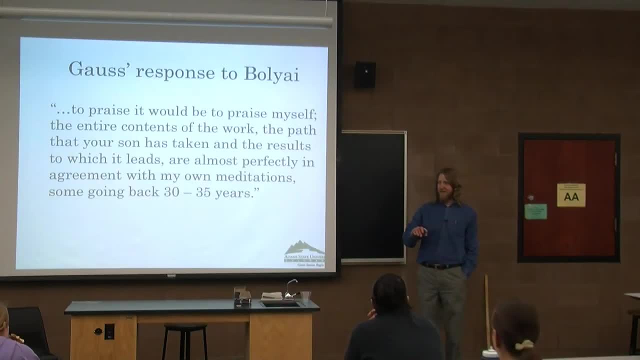 By the way, in Gauss' defense, history has supported his position. He did not publish his results, but after he died they were going through his papers and what do you know? he did come up with all of this stuff before wrote it up and 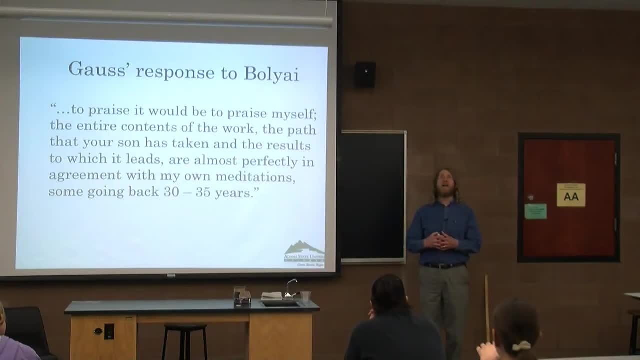 said: hey, this is pretty neat, But he said that he feared the outcry of the world, The outcry of the, the outcry of the dullards- I think is the way he said- if he were to publish these because the results are so weird and counterintuitive. okay, 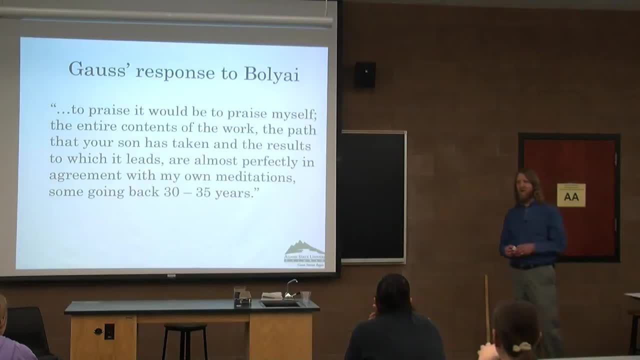 Well, as you might imagine, this didn't sit very well with the young, younger Bolyai. He was convinced that Gauss was lying. He was convinced that, no, Gauss didn't think of this. he's going to steal my ideas. and it turned Janusz Bolyai off to mathematics and he basically gave up mathematics and never. 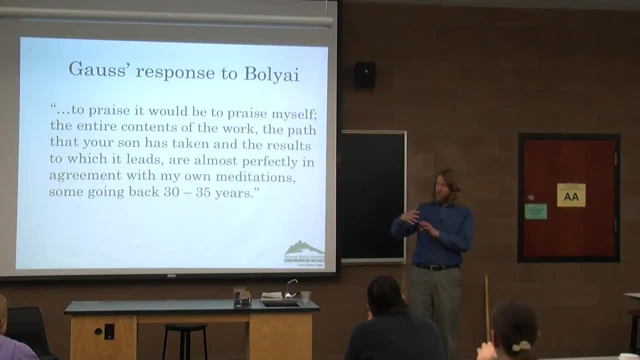 never really did anything else. His results, his which we now know as non-Euclidean geometry, were published as an appendix to a geometry textbook that his father published some years later. okay, But he never in his lifetime got the well, the notoriety he should have got the credit. 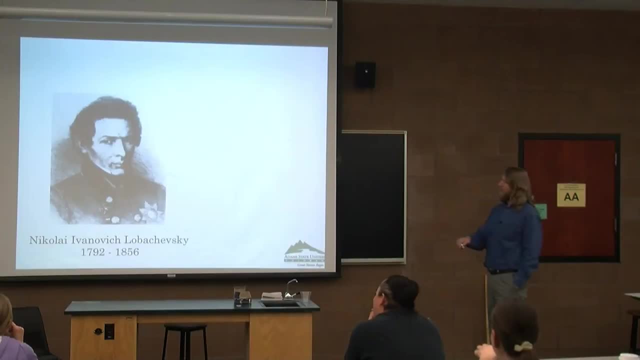 that he should have Now. I should mention here that about the same time Bolyai was doing this, a Russian mathematician named Nikolai Ivanovich Lobachevsky- That's a great name, It rolls off the tongue very well- Came up with many of these same results in about about the same time, about 1829. 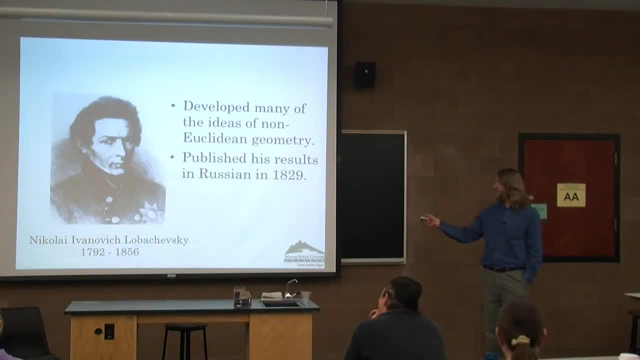 So why does? why was he not noticed for it? Well, right there, He was published in Russian. Nobody was reading Russian, okay? So it languished in obscurity for many, many years until eventually it was translated into other languages and people said: oh wait a minute, Lobachevsky was all over this. 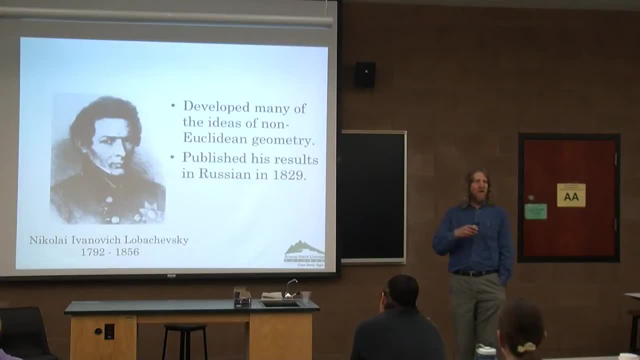 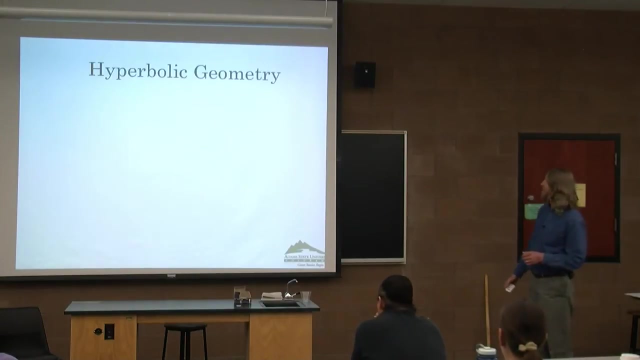 And so now, if you look up the founders of non-Euclidean geometry, Most textbooks give Bolyai and Lobachevsky equal credit for developing this non-Euclidean geometry. Okay, Well, let's talk about the non-Euclidean geometry, since that's what we're here for. 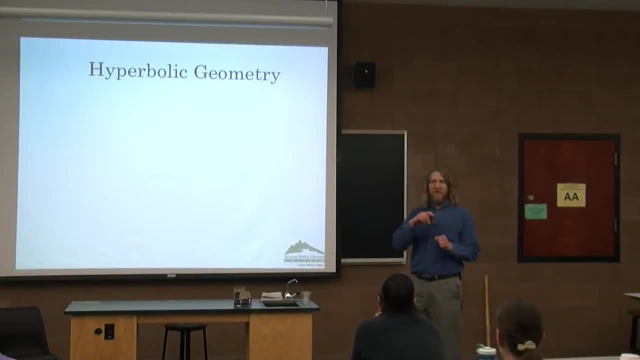 If you take the first negation of that parallel postulate that there are no, excuse me that there are more than one line through the given point that's parallel to the given line, then you wind up with something called hyperbolic geometry. 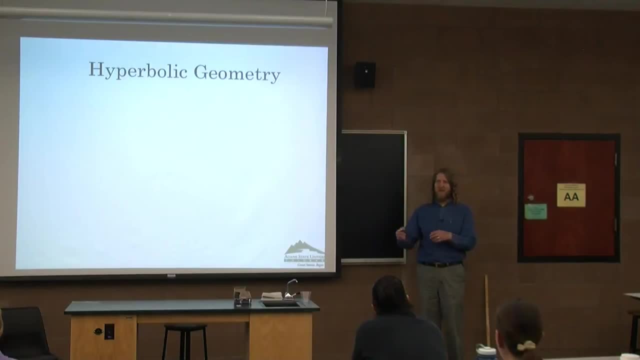 Or Lobachevskian. I've seen it Gaussian-Bolyai-Lobachevskian- okay, But most folks would just call it hyperbolic, okay. So what happens? is that the most common model that you see? well, okay. so, as we said, there's. 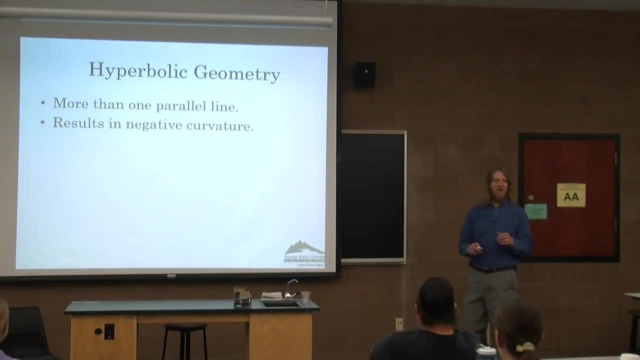 more than one parallel line. it results in the space having what's called negative curvature, And I have a picture in a moment that I'll show you what negative curvature means. okay, But the other bizarre result here is that triangles then have an angle sum less than 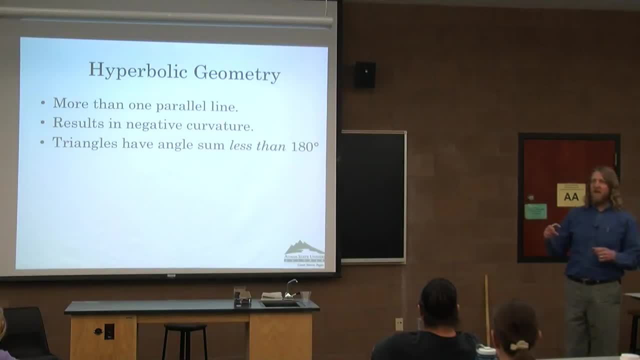 180.. And perhaps even more disturbing, the sum of the angles in a triangle is not fixed. okay, It depends on the size of the triangle. okay, They all have angle sum less than 180, some more so than others. In fact, if you take 180 and subtract the angle sum, that's referred to as the defect, 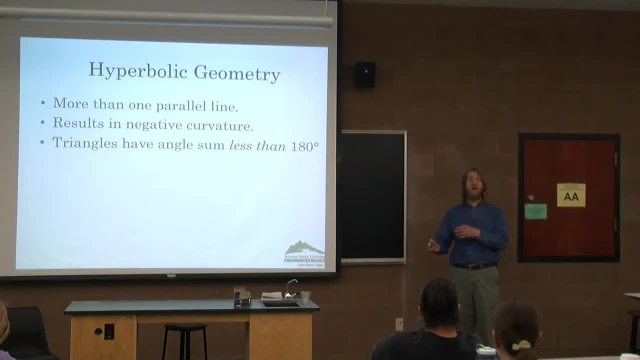 of the triangle, And you can make a statement that the larger the triangle, the larger the defect, And I'll show you some pictures of that too. As far as negative curvature, well, most folks visualize these things on like a saddle. 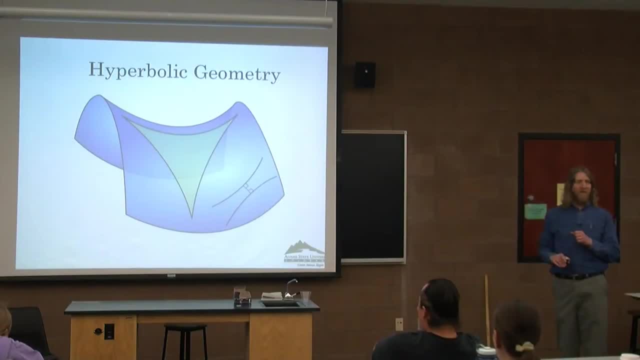 And this is actually a slice of a hyperbolic, paraboloid, Okay, But it kind of looks like a saddle, right, You can imagine sitting on it. And here you can see this triangle on this surface. And this triangle- well, I mean the curvature of the surface bows the sides in so that the 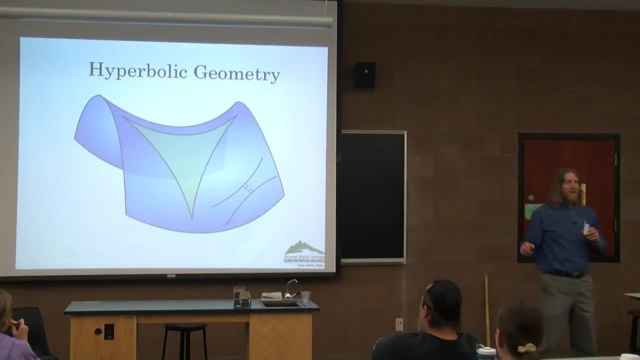 angle sum turns out to be less than 180,. okay, Now this again, this is negatively curved, and probably the easiest way I can explain that Is: imagine yourself standing up here at the apex of the surface. Okay, On the saddle. 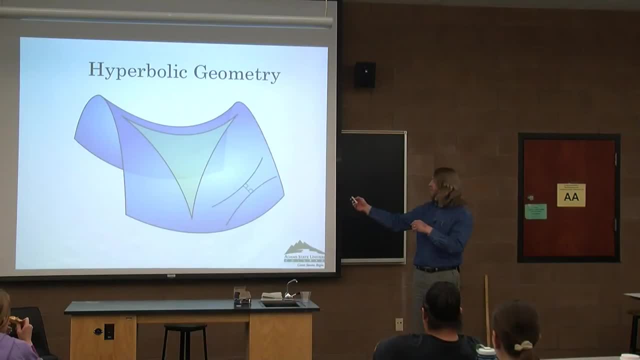 Okay, And facing what we'll call the front of the saddle, And what you would find is that the thing is curved upwards, right, It's concave up in this direction and concave down in that direction. Okay, And the problem with trying to use this as a model for your hyperbolic geometry is if 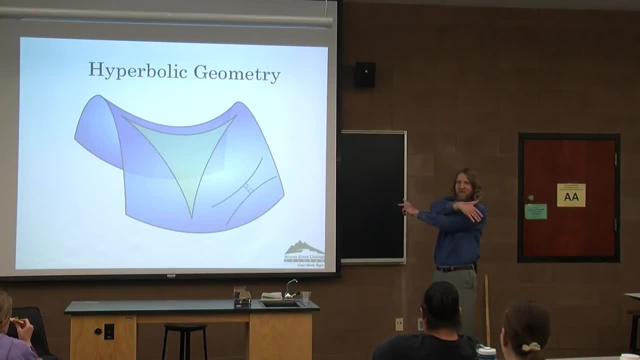 you try to extend it, eventually the thing winds up intersecting itself, Okay, And then things get ugly and hard to see. Okay, But So there is another model. the most common model that you see of the hyperbolic geometry is due to the mathematician Poincaré. Henri Poincaré came up with this disk model. 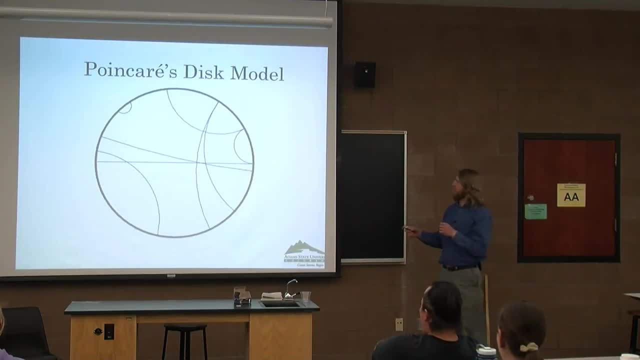 Okay, Now this one takes a little bit of explaining. What you see here is: this is the whole of the space. Okay, This is all there is. This thing does not extend to infinity. It in fact does not even include the boundary. 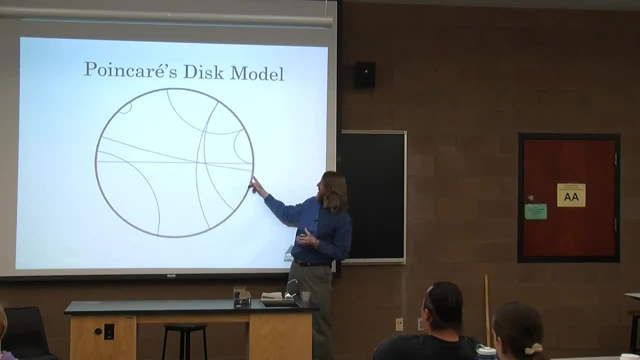 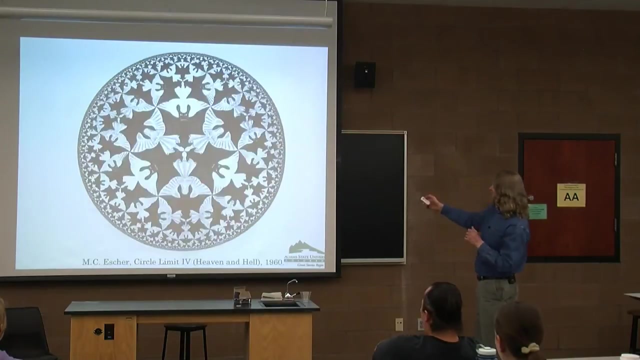 Okay, This is actually an open disk, Right? It does not include the boundary And lines. lines in this geometry are defined to be the arcs of circles that are perpendicular to the boundary of the disk. Okay, Geodesics is another term for it. 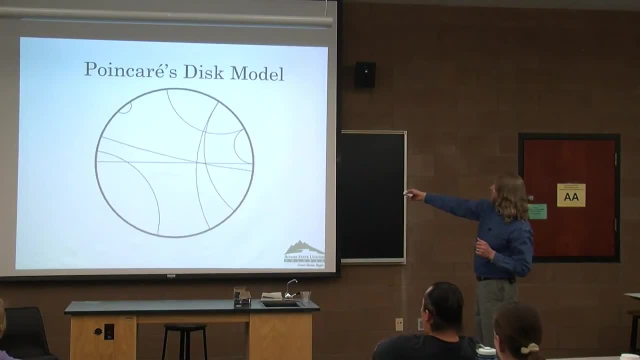 Whoops, Hello, Wrong button. Okay, So you see that this is the arc of a circle. I mean it would continue out here, but of course that's outside our disk and we don't care about that- And it's perpendicular to the boundary here and here. 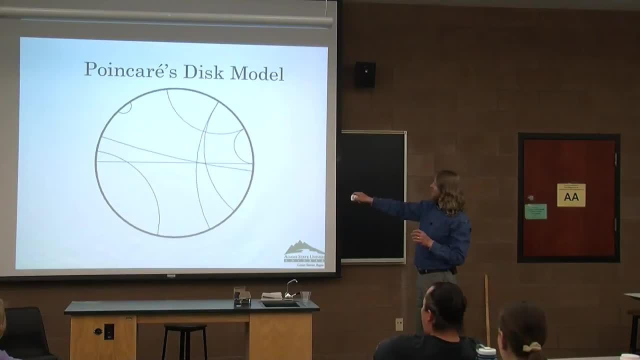 The one exception. the other type of line is: well, what happened? you can also have a regular, regular, regular line that goes through the center of the disk. Okay, So lines in Poincaré's disk model come in two flavors. 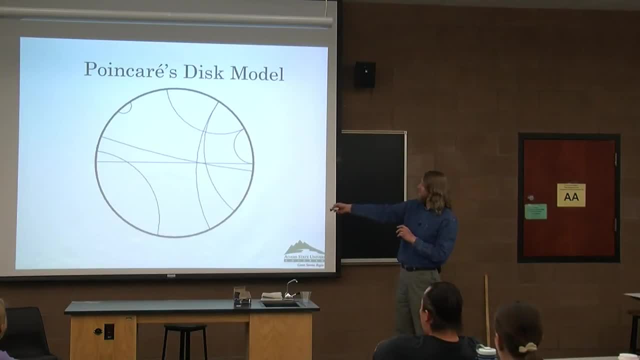 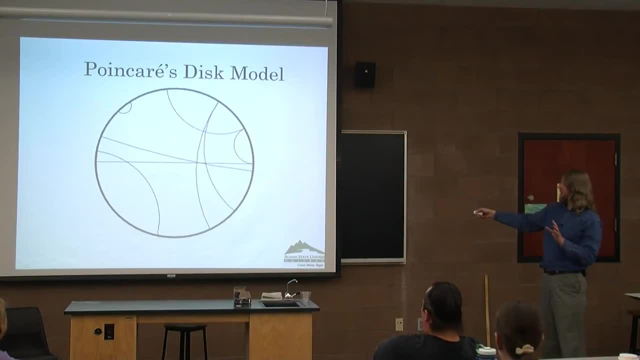 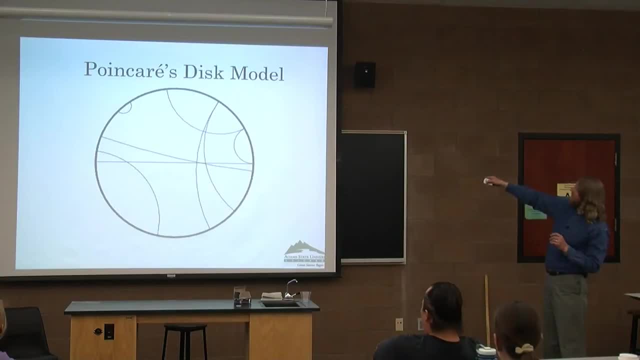 this circle here, right, would probably be right around here somewhere. So just let that center run off to infinity, Okay, And then the thing flattens out and that's how you get the lines that are actually through the center. Now this shows us a lot of neat things. One thing it shows us is the multiple parallels, Because you can imagine: imagine this is your given line L and imagine this is your given point P, not on L, And what you see is that here are one, two lines through P that do not intersect L. 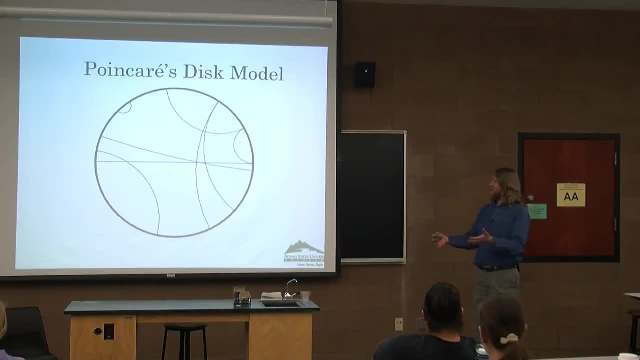 And of course, it's also easy to see that once you open the door to two parallels, you actually get infinitely many from that. So yeah, One thing that's not obvious in this picture with the Poincaré disk model is distances. 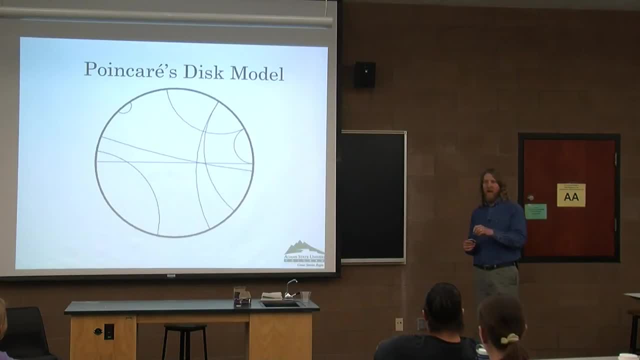 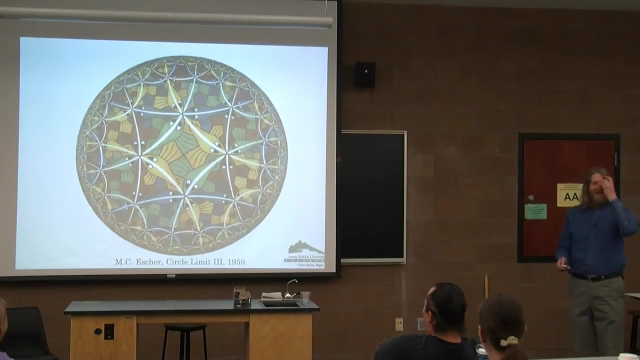 Because the distance actually is not fixed here. In other words, the distance between two points gets magnified out here toward the edge. All right, The best picture I've found is MC Escher, And this is perhaps the Poincaré disk model was the motivation for Escher's picture here. 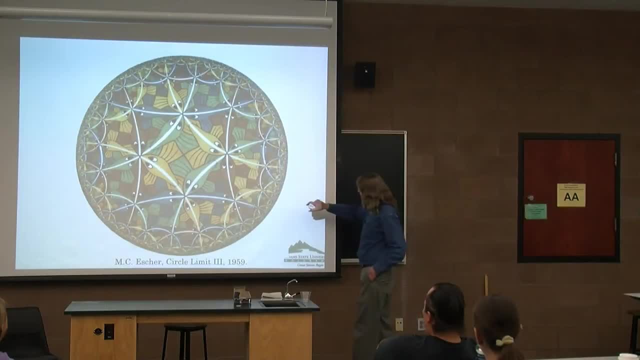 But if this were really in the Poincaré disk model, then this little fishy right here is exactly the same size as this one. Okay, Because of the way the distance is defined in the Poincaré disk model, All right. 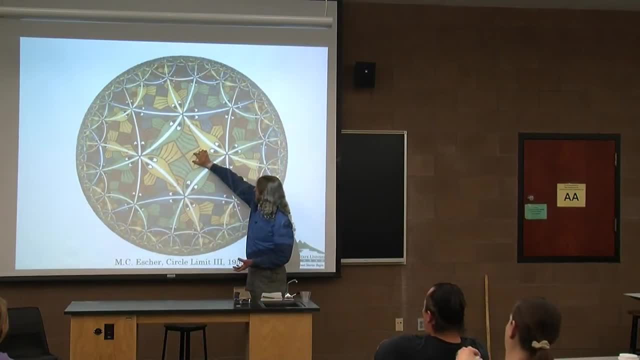 In other words, if I measure this as being, you know, like three inches there, then it's going to be the same size as this one. Okay, It's. you know 270 feet here, or something like that. And if you think about okay again- we generally don't use this word in geometry class- 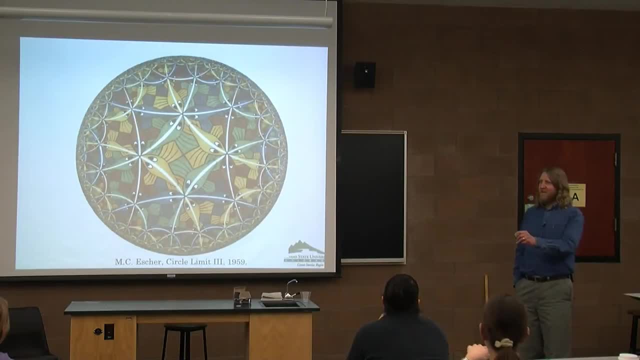 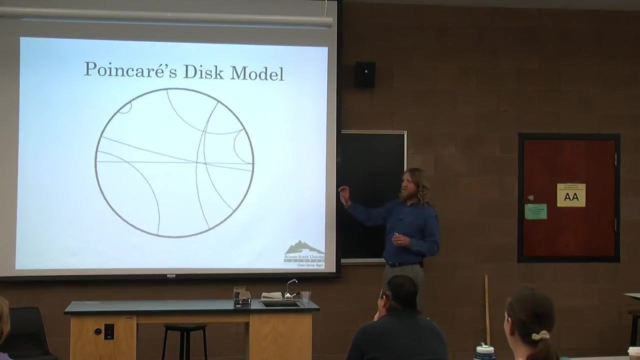 But you think about straight lines, okay, And you talk about- you've heard people say the shortest distance between two points is a straight line, Okay, And every mathematician in the room cringed when I said that, Okay, But you can see that here because, remember, the distance function isn't fixed. 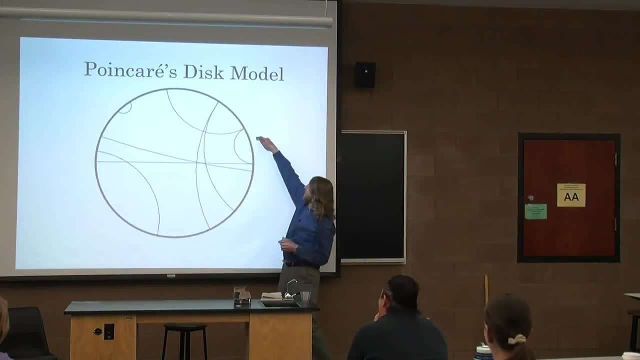 Right, It gets magnified out here toward the edge. So if you're going to try to go from, say, this point to this point, what's the fastest way to get there? Well, if you move along here, then the distance function is so huge that might be, I don't know, trillions of miles. 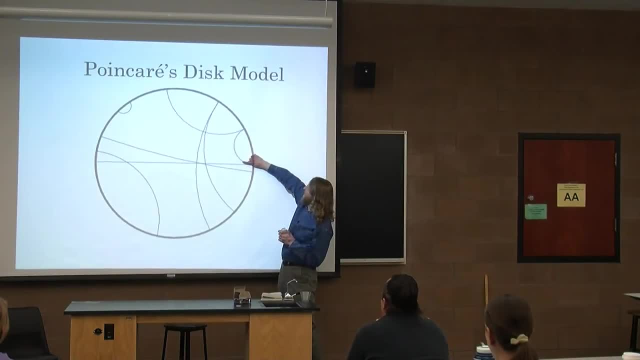 So what's the best thing to do? The best thing to do is to come perpendicular to that, come out and then swing around like that. So that is actually the shortest distance between those two points. is following that peculiar thing? Okay, Just another picture of MC Escher. 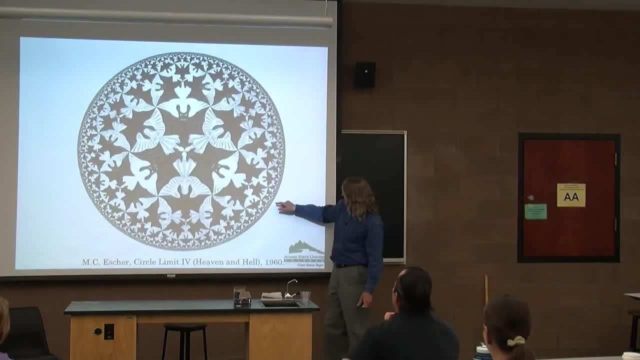 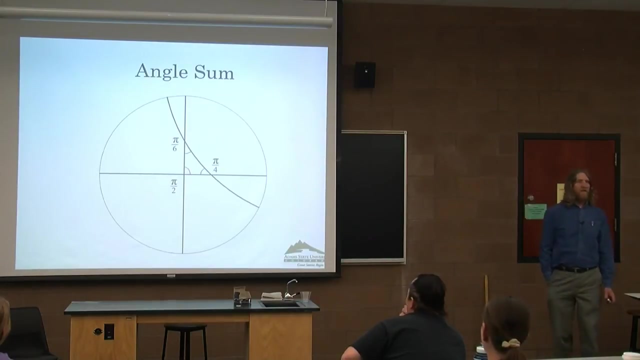 And again, remember the weird thing with the distance means that this bat here is the same size as this bat here. Okay, That's the Poincaré disk model. What about these triangles? Well, this is a triangle in the Poincaré disk model. 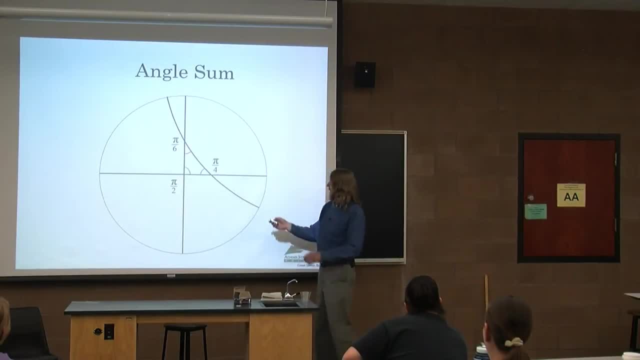 You notice, two sides of the triangle have been formed by lines that go through the center, And then the third one is out here. Okay, And unfortunately- or maybe fortunately- The angle measures here are given in radians instead of degrees. What's the sum of the angle measure of this triangle? 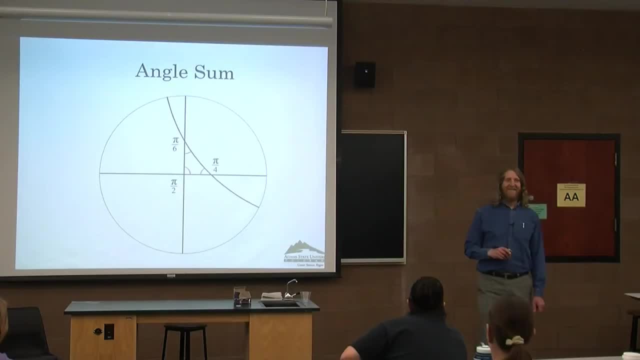 11 pi over 12.. How many degrees is that? Okay, It turns out that's 165 degrees. Okay, So here you have a triangle, right, And of course, the triangle stops at these three points. It's just that this picture that I lifted off the Internet didn't 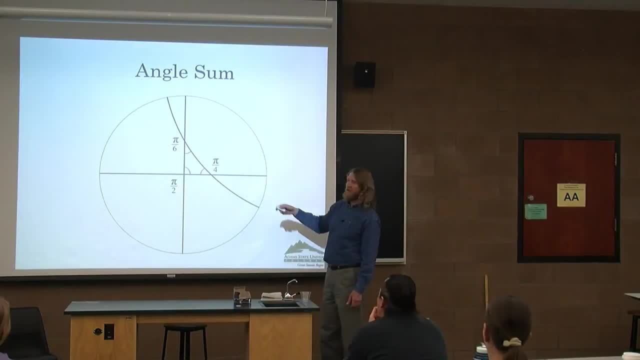 Okay, You find that the sum of the angles inside this triangle is 165 degrees, not 180 degrees. Okay, And the bigger you make this triangle, the greater that defect will become. Okay, Is that? Yeah, I think that's right. 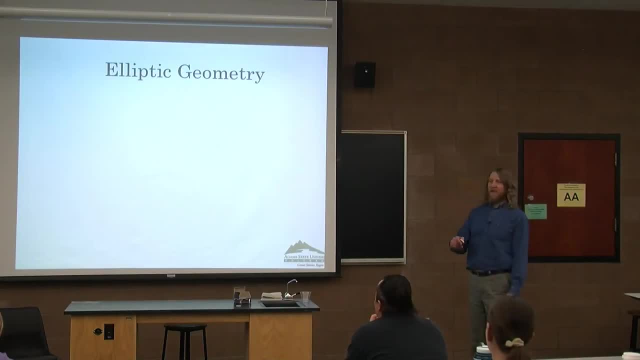 I hope that's right. Okay. Next, If, on the other hand, when you negate Playfair's postulate, you make the assumption that there are no parallel lines, you wind up with something called elliptic geometry. Okay, No parallel lines. 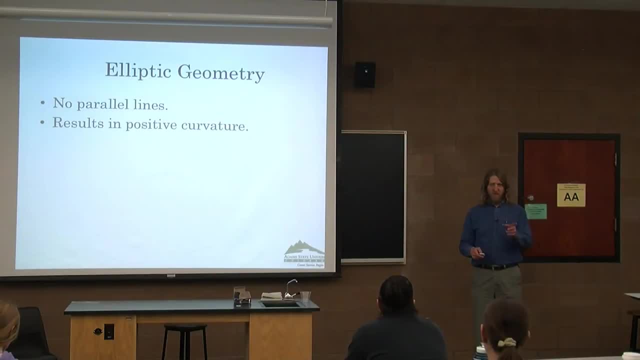 And it results in positive curvature of the space, which I will show you an example of in a moment, And, of course, the fact that the triangles have angle sum that's greater than 180.. Okay, Now I need to issue a disclaimer here. 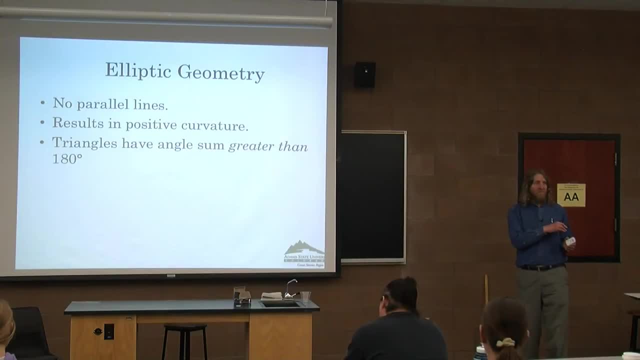 because I'm about to show you an example, a model of the geometry which has some technical problems. There are some technical things that you need to address when you do this. no parallel lines, because that turns out to inflict with some other things. 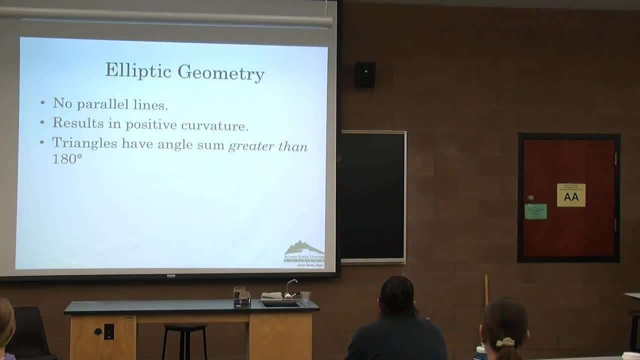 But they can all be patched up And this is a good model, because? well, because it's easy to visualize, Okay, And so it's called spherical geometry, for obvious reasons: It's geometry on a sphere, And I happen to have a sphere. 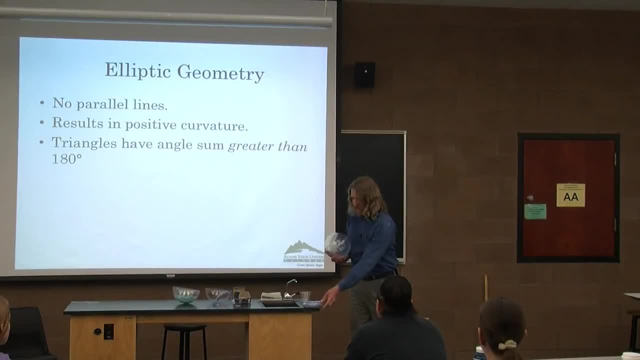 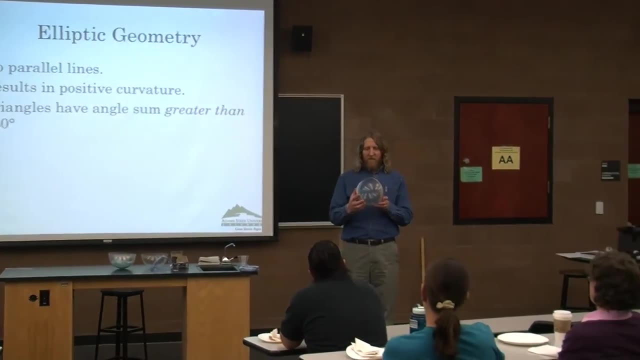 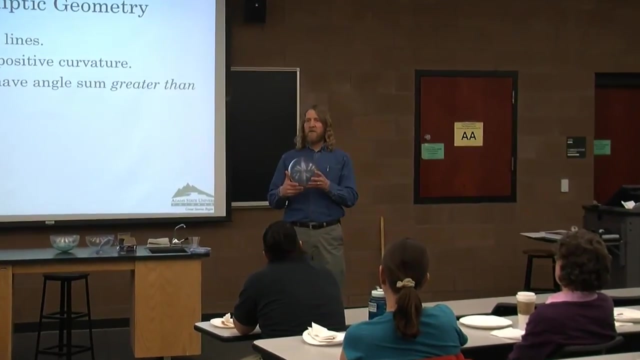 Okay, So here's the sphere, And so the question then becomes: what do we consider to be lines on the sphere? And well, for a variety of reasons, It turns out that lines on the sphere then get defined as what are called great circles. 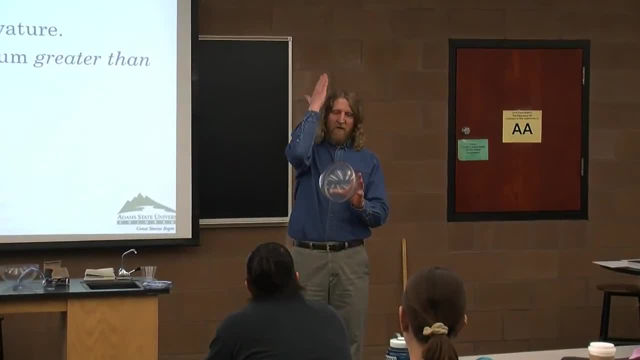 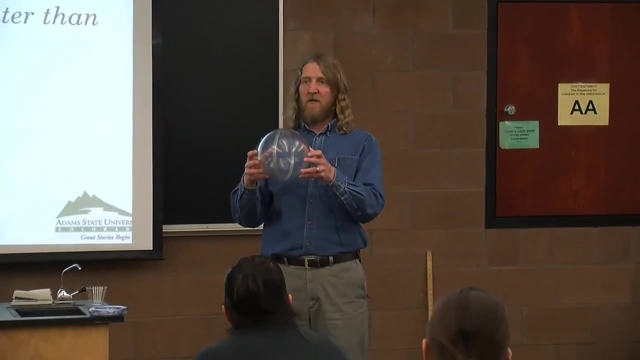 Okay, A circle. in other words, it's what happens if you cut, if you take a plane and pass through the center of the sphere, where it traces the surface of the sphere. that's a great circle. So, for instance, the equator is a great circle. 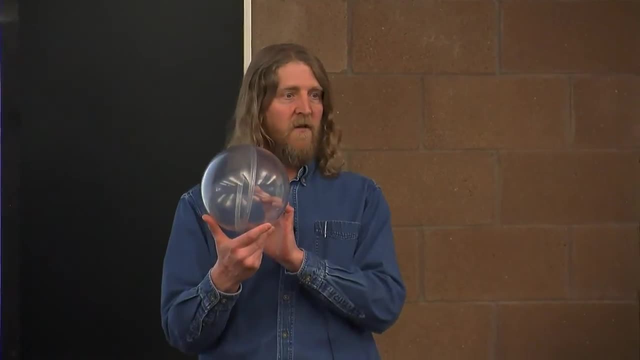 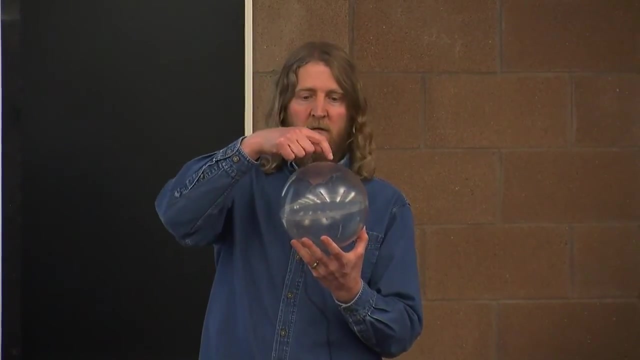 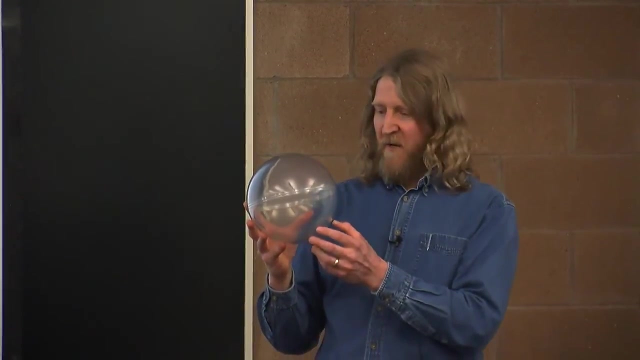 All lines of longitude are great circles, Okay, But none of the other lines of latitude are great circles. Right, The arc circle or the arctic circle is not a line, strictly speaking, Neither is the tropic of cancer or any of those things. 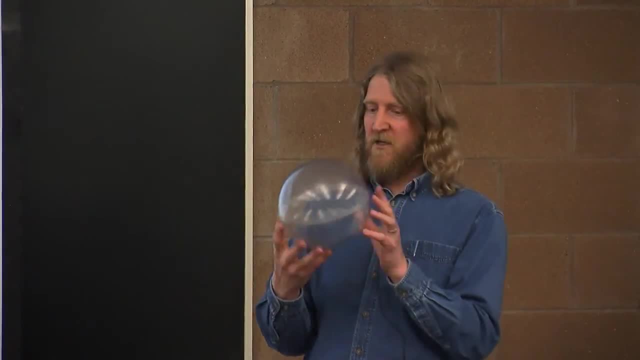 Okay, Just the lines of longitude and the equator. Of course, you can do this anywhere, And this came with a handy-dandy thing for drawing lines, And so here's a ruler. You want to draw a line on this sphere? 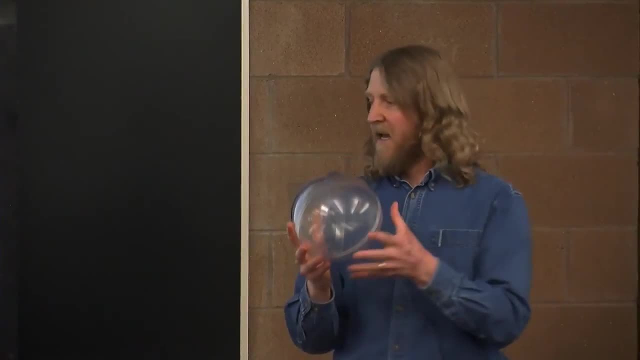 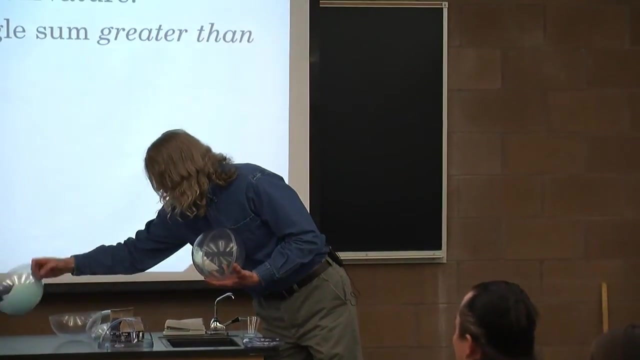 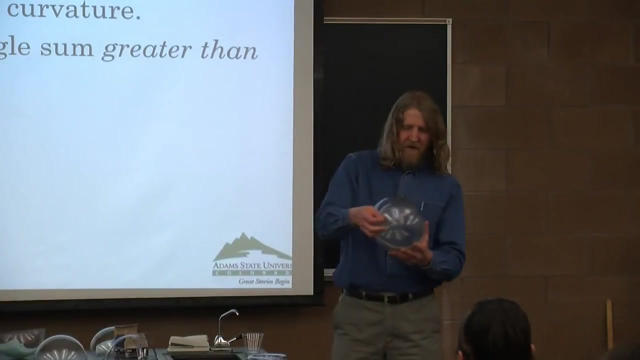 You put your little ruler on there and you draw it around. Okay Now, so let's talk about triangles. Triangles, Because I have here. aren't these great? They look like big contact lenses. So what I have here is I have drawn three triangles on this surface of this sphere. 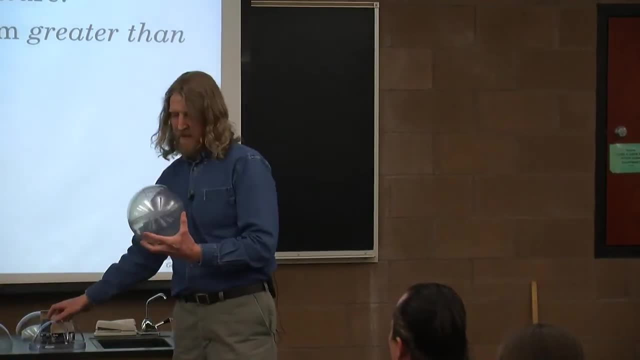 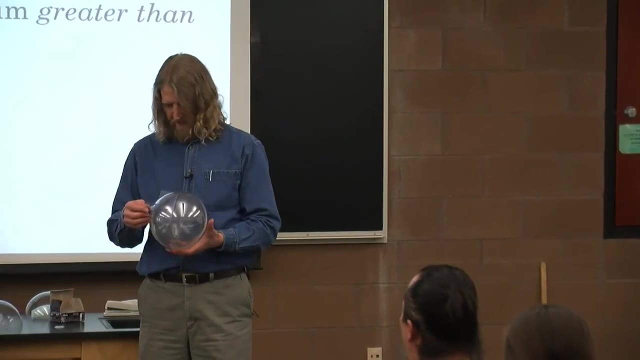 Okay, And each one of these lines- okay, well, segments- actually is indeed a portion of a great circle. This thing isn't fitting on, It's not squished on enough, But So I use this. 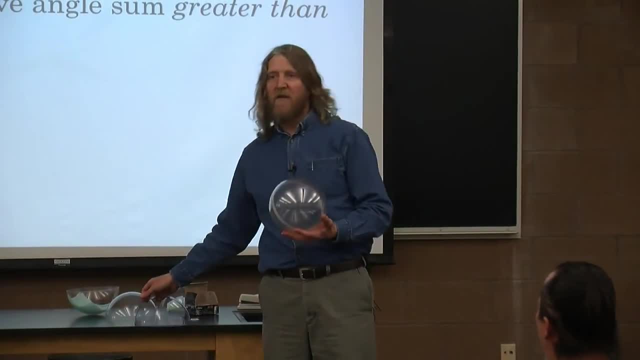 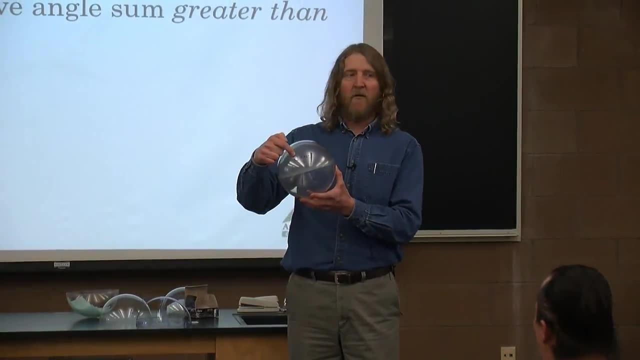 I drew it out three triangles, and then I measured the angle sum roughly, Okay, And what I found was that this little guy here had an angle sum of about 183 degrees. Okay, I made it a little bit bigger. I came up with one that had an angle sum of about 191 degrees. 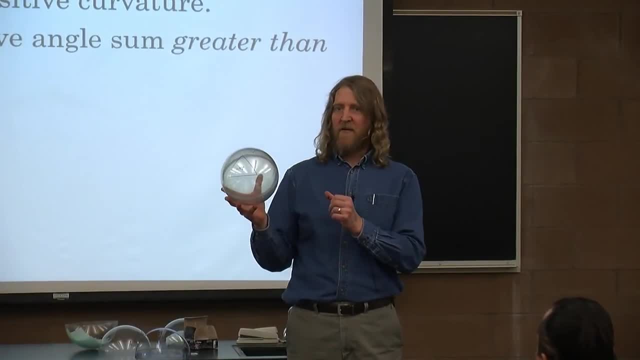 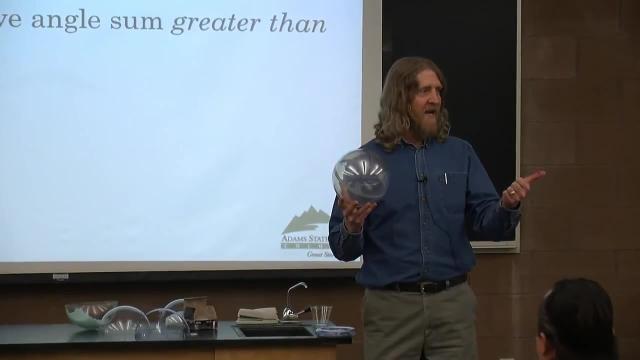 Still bigger. I came up with one that had an angle sum of 193 degrees. And so you see again this property, that not only do they have angle sum greater than 180, but they don't have an angle sum greater than 180.. 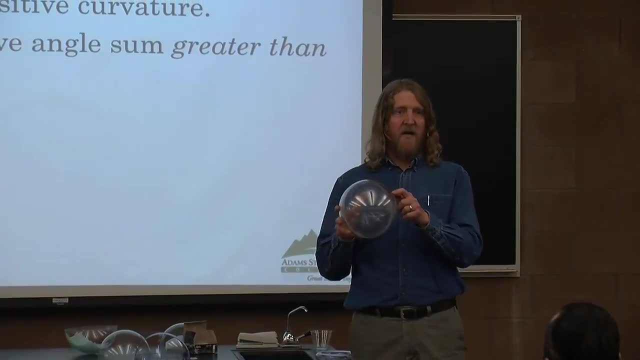 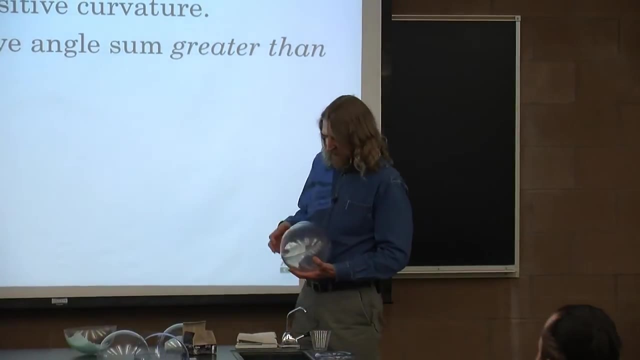 They don't have the same angle sum And in fact, the larger you make the triangle, the larger the angle sum becomes. Okay, And in fact what you can do is you can take this to an extreme, kind of a ridiculous extreme. 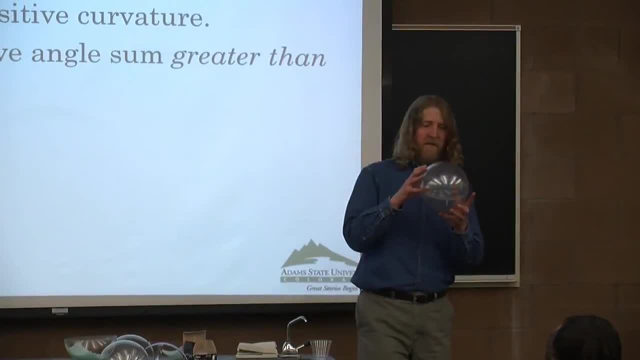 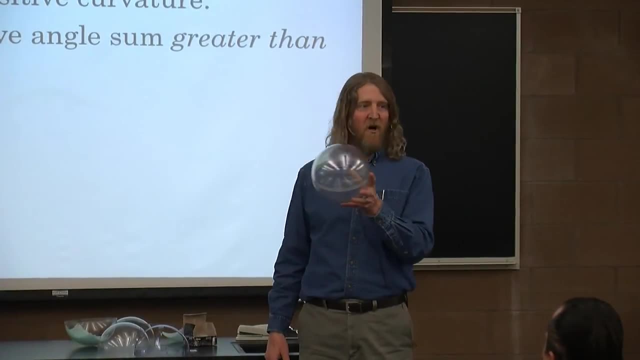 and you can make this triangle. This triangle has an angle sum of 270, and in fact is an equilateral right triangle. Okay, Because all three angles are right angles in this triangle Has an angle sum of 270. Um. 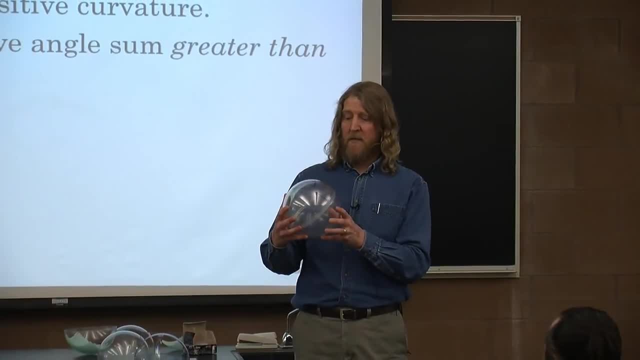 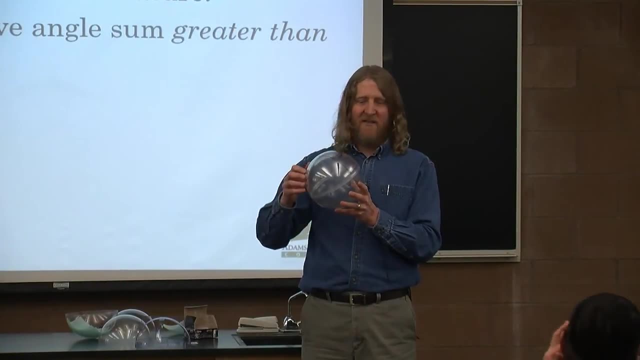 What's the maximum you can have? To be honest, I'm not quite sure, Because things get a little bit weird. Remember, I told you there were some technicalities we had to address for the other postulates And at some point, if you take this too far around, 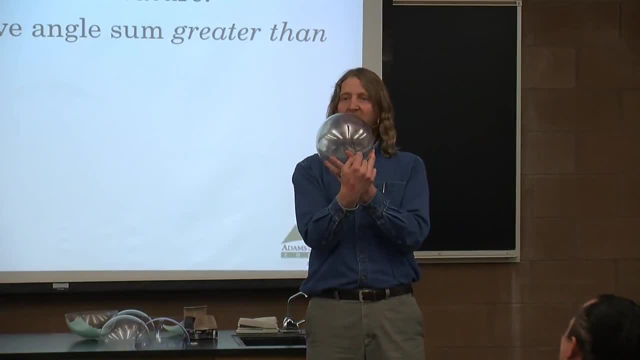 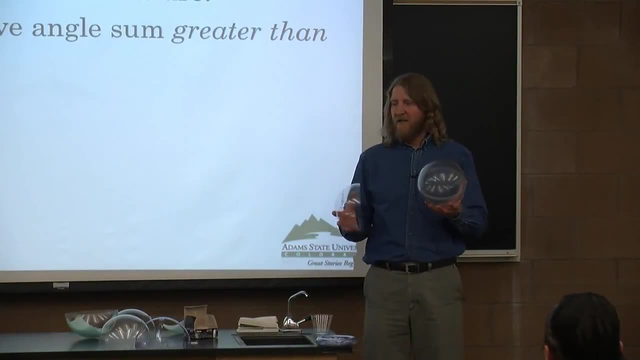 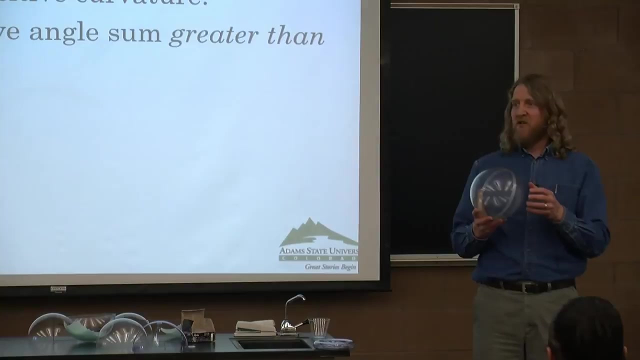 then you shouldn't be drawing your triangle this way, You should be drawing it that way, And so, anyway, Now this isn't just purely an academic exercise, because it has a real-world application. Okay, Remember, I talked about how a straight line is the shortest distance between two points. 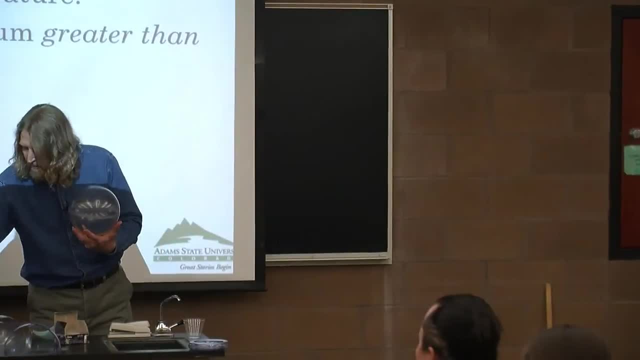 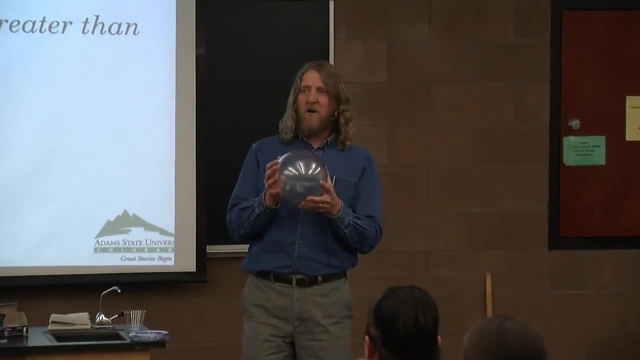 So suppose that you were going to take a flight from, oh, I don't know. let's say you were going to fly from Chicago to Rome. Okay, Now, Chicago and Rome are both located at about 40 degrees north latitude. 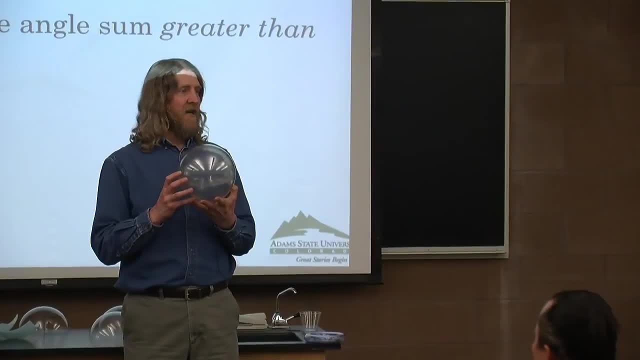 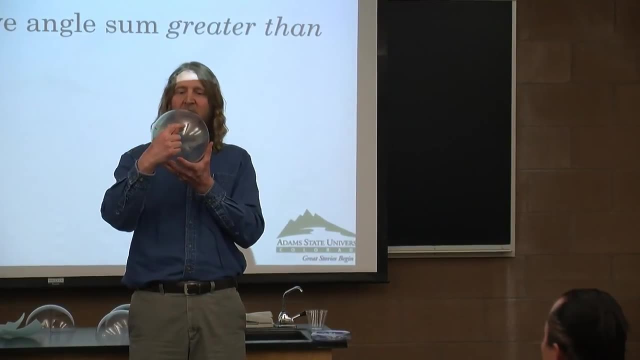 Okay, And so you would think that if you go and you take your non-stop flight from Chicago to Rome, you hop into the plane and he flies along the 40-degree north latitude and flies over here to Rome. But that's not what they do. 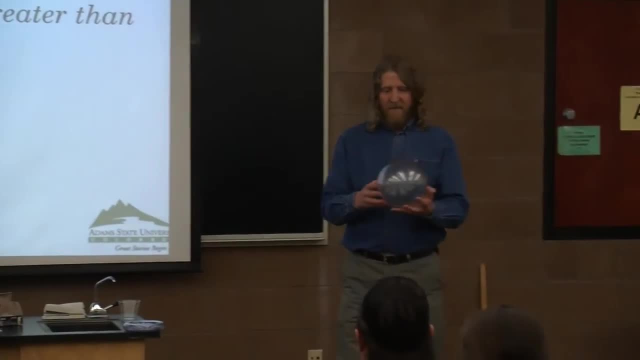 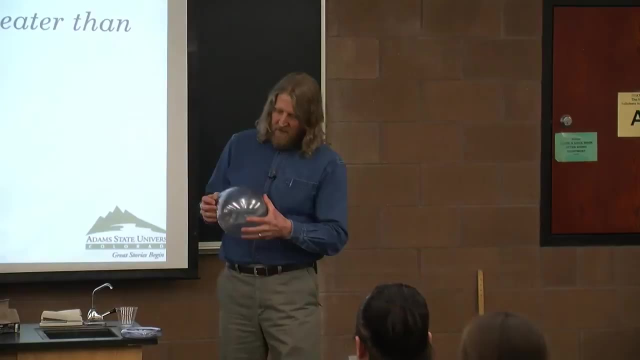 Some of you are shaking your heads. You know what they do. What do they do? Well, maybe What they do is they fly along the path of a great circle, which you can see. the great circle that connects Chicago to Rome looks about like that: 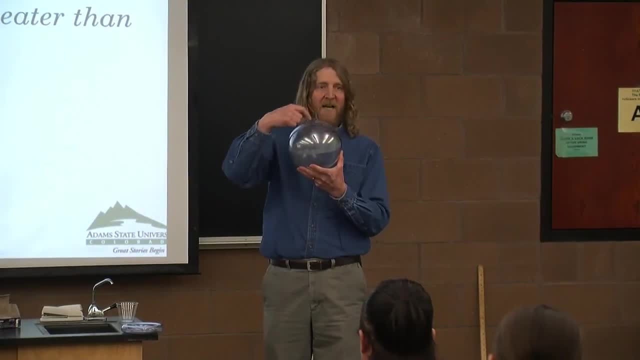 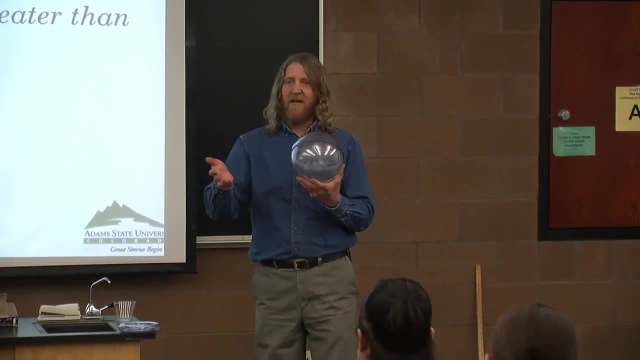 So it actually flies north and then over. Well, it's actually flying there. It's flying there by the shortest distance, Okay, Which is. and so the shortest distance then from Russia to the United States does go over the North Pole. 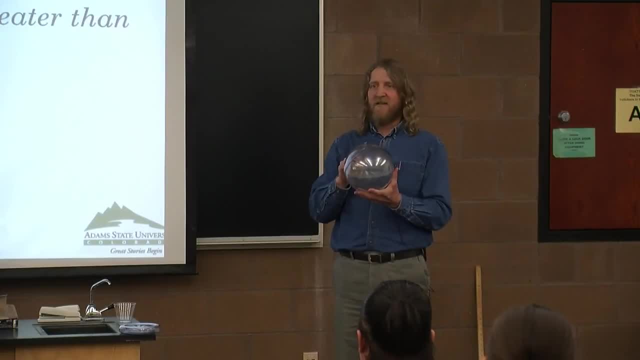 And that's why we had all those during the Cold War, all those early warning missile sites up there, Because when you wanted to go from one side of the globe to the other, you didn't go this way, You go that way. 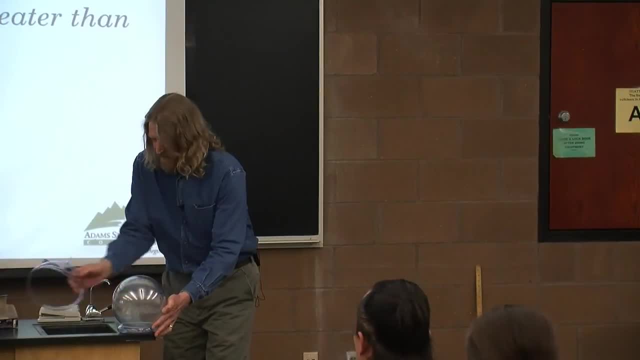 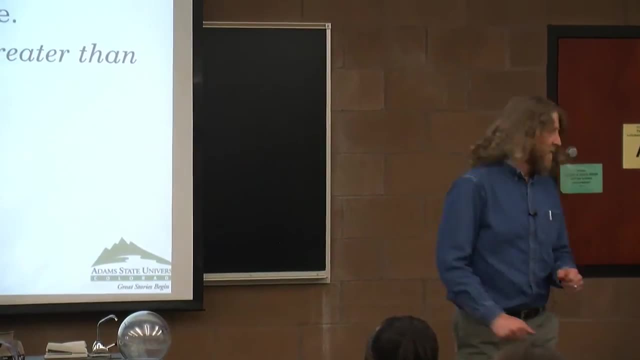 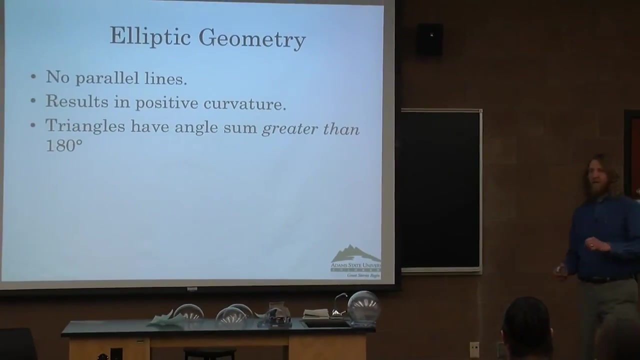 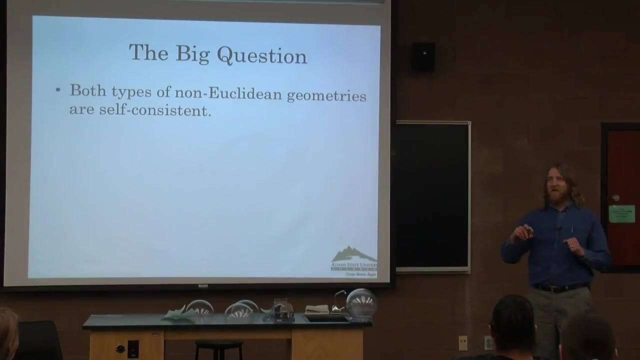 Okay, And so it's not just an academic exercise. Okay, Spherical geometry: How much time do I have left? Okay, Good, All right. So now the astute observer will note that up to now, we found both of the types of non-Euclidean geometry are self-consistent. 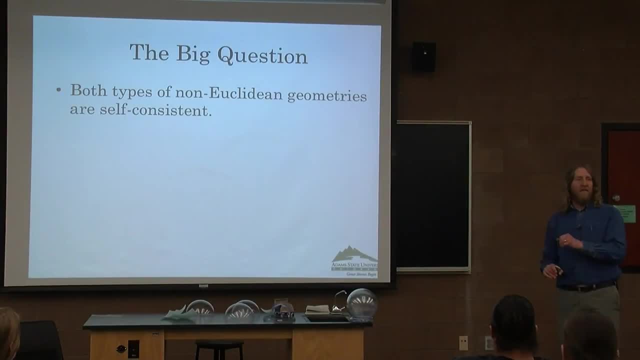 Again with the elliptic one. there are some technicalities that have to be addressed, But you can address those and you can make that completely self-consistent. Now, what do I mean by self-consistent? I mean you cannot prove a result that contradicts an already proven result. 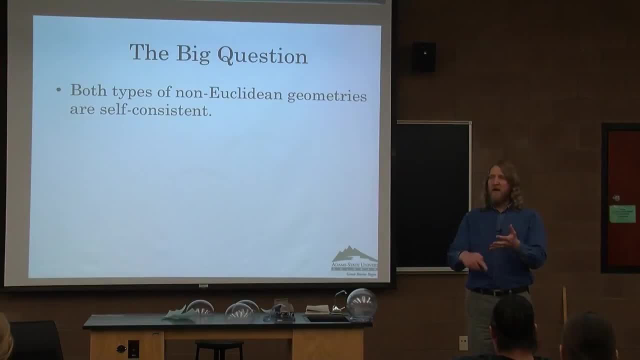 Okay, You don't have any contradictions built into it. So both of the non-Euclidean geometries are self-consistent. Euclidean geometry, of course, is self-consistent, But they are also mutually exclusive. Okay, You cannot have a space that is Euclidean and non-Euclidean at the same time. 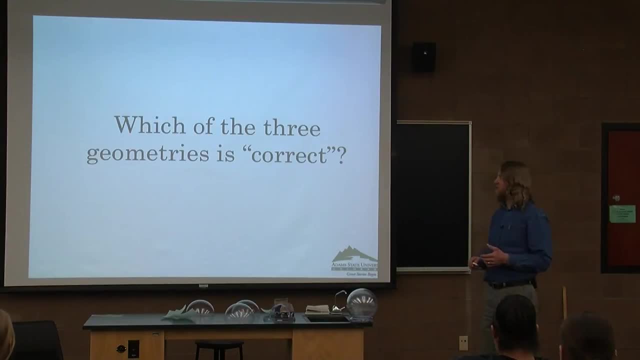 But we live in a space, And so the big question, then, is which of these three is correct? Which of the three geometries actually represents the geometry of the universe as we know it? Well, how could we figure this out? Well, one thing we could look at is we could look at triangle differences. 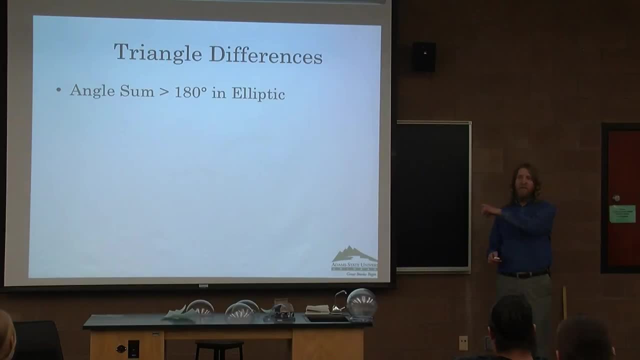 Okay, Because, remember, we said that the angle sum in elliptic geometry of a triangle has to exceed 180.. Whereas in Euclidean geometry it's exactly equal to 180.. In hyperbolic it's less than 180.. So it seems like all you have to do is build yourself a triangle, measure the angles and then you can figure out. 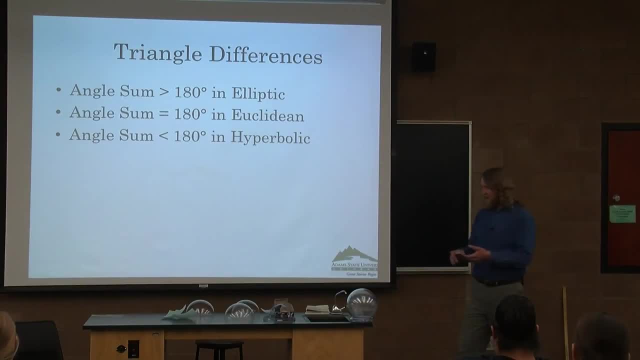 Is it 180?? Is it bigger? Is it smaller? Okay, Well, if this has taught us anything, it's that if space is non-Euclidean, then you're better off using a big triangle to try to measure it, Because small triangles get too close to 180. 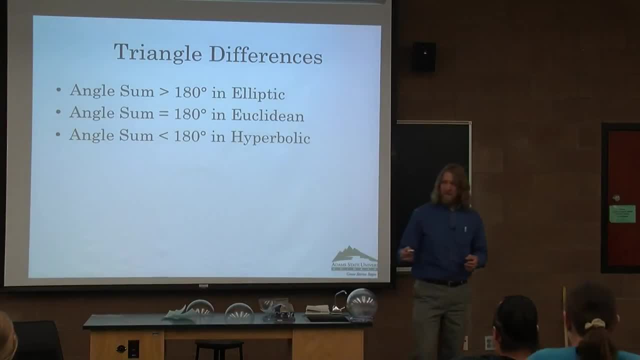 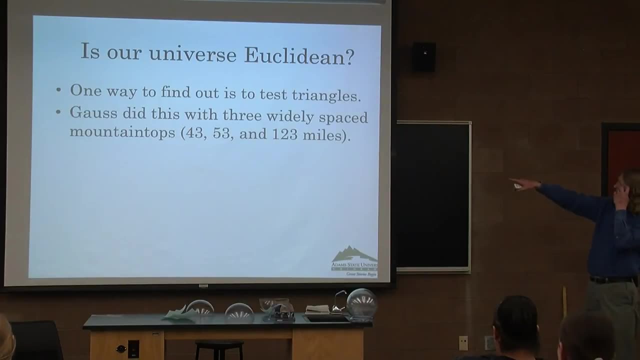 So our old friend Gauss in the 1800s did this. He found three mountaintops. Okay, That, Basically he wound up with a triangle that had side lengths of 43 miles, 53 miles and 123 miles. 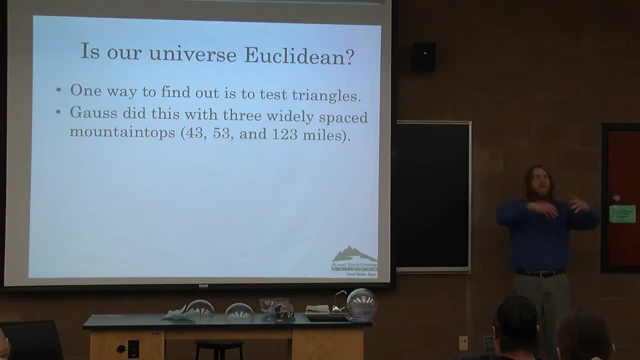 Okay, And he had teams of people go up onto each one and make a big bonfire And they measured these angles, Okay, And they measured the distance. They did everything very precisely And guess what they came up with? Guess 180.. 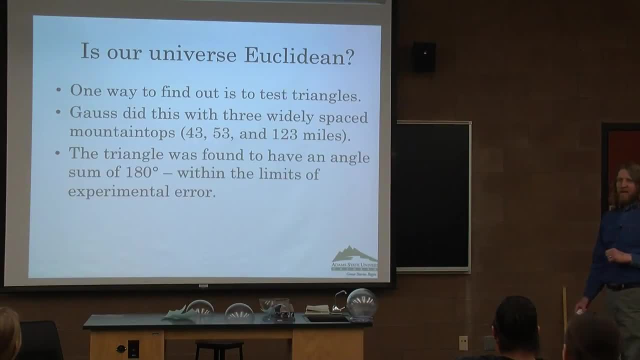 180.. Exactly, But within the limits of experimental error. So it was actually 180.. So it was actually 180, plus or minus a little bit. So what did he prove? Nothing, Nothing. And now here's a weird logical twist about this, though. 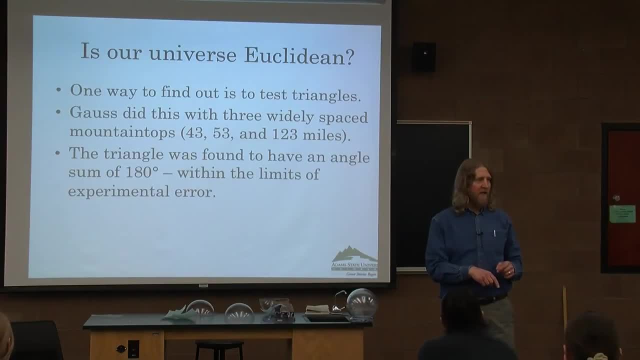 If the universe really is Euclidean, there's no way you could ever prove it by measuring triangles, Because you'll always have some experimental error. So I mean you might get it out to 7,, 8,, 10 decimal places. 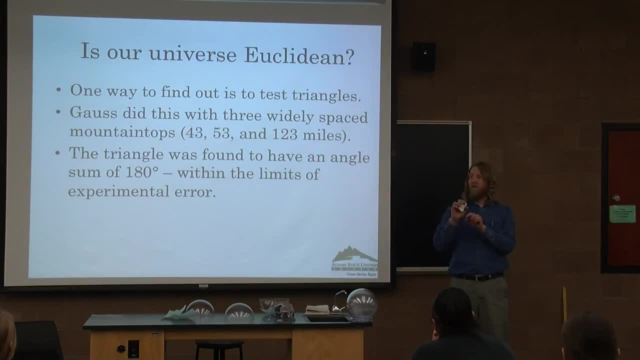 But there's always going to be that little plus or minus, So it might actually be a little bit more than 180.. It might actually be a little bit less. However, if space is actually non-Euclidean, then you could prove that by using triangles. 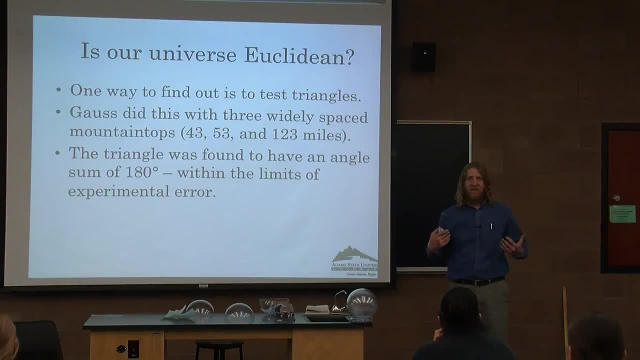 Okay, Because, say, for instance, you measured your triangle to have an angle sum of 183 plus or minus 1.. Well then, by golly, you know it's more than 180. And you know you have to be in the elliptic geometry case. 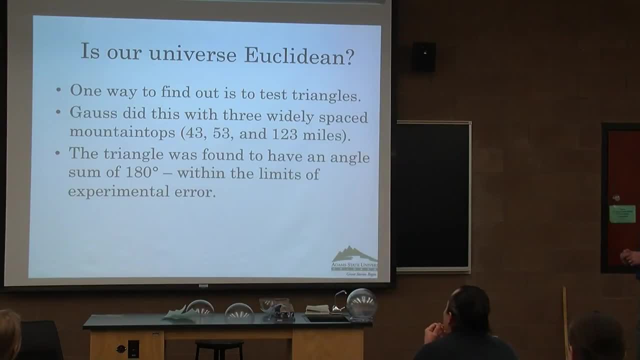 All right. So that was a bit disappointing, And there are folks who claim that that's not what Gauss was doing. He wasn't trying to prove it. He knew you couldn't prove space was Euclidean this way. Well, it seemed like a lot of trouble to go through if he wasn't trying to prove it. 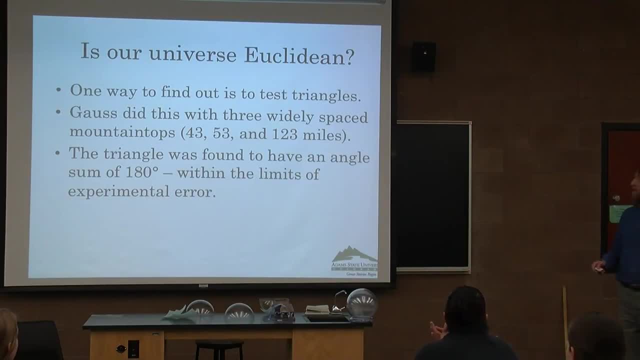 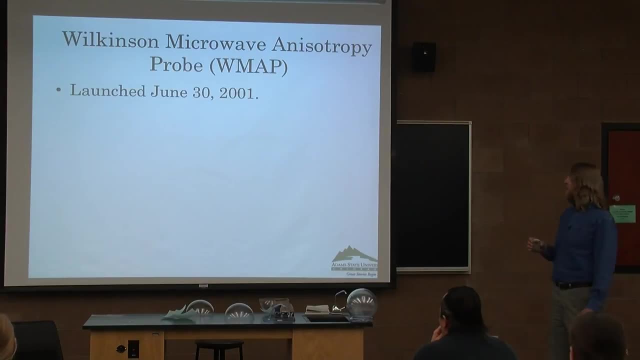 There have been more recent attempts. In June 2001,. NASA launched a probe called the Wilkinson Microwave Anisotropy Probe. Anisotropy, Anisotropy, Anisotropy- Okay, All right. And this measures? it takes detailed measurements of what's called the cosmic microwave background. 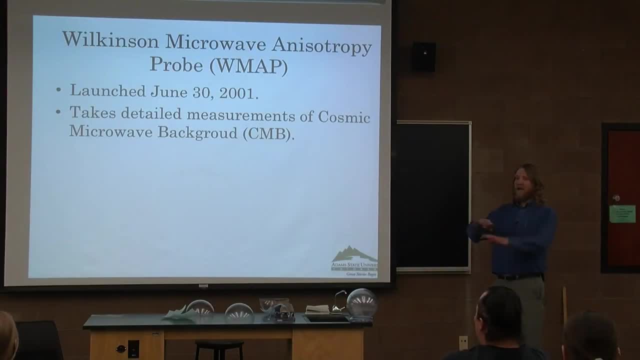 Essentially, as I understand it, it's the leftover radiation from the Big Bang And it looks at how it's distributed And according to the theory of relativity, if it's at this range, then the space would be Euclidean. it would be non-Euclidean. 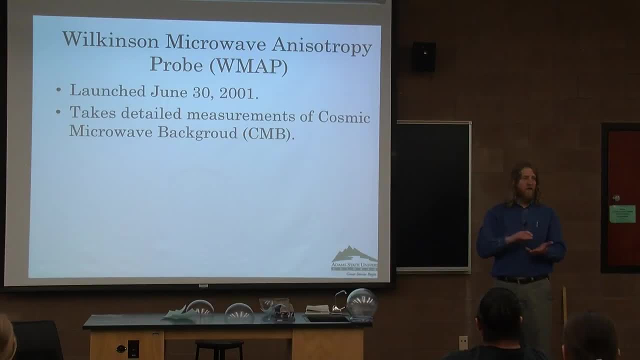 So they managed to measure the curvature of the universe. Okay, And as of, I think it was December of 2012.. The latest, best data from the Wilkinson Microwave Anisotropy Probe shows that the curvature of the universe is: 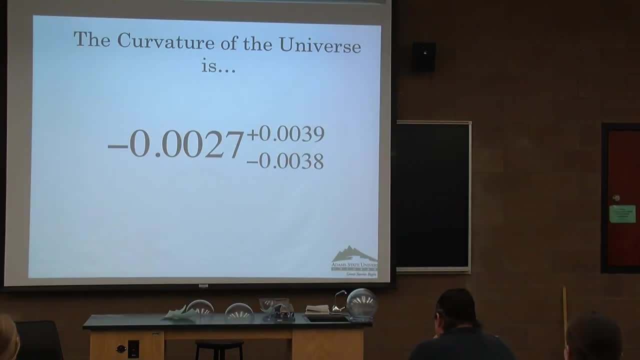 So what's the answer? We still don't know. Okay, If it is hyperbolic, okay, if it is hyperbolic, it's not very much hyperbolic. I mean, this isn't a very large number. 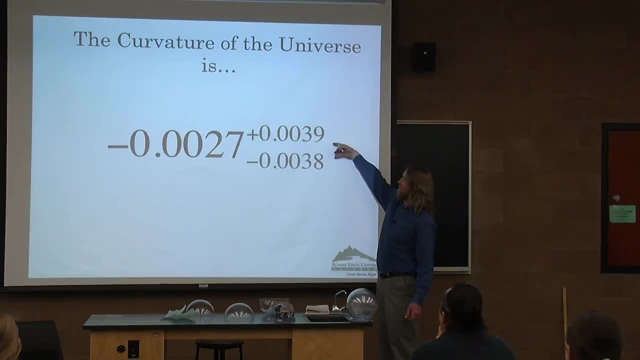 It's a very large negative curvature And, of course, zero curvature is still within the range of error here. So the best guess at this point in time is that the universe is probably Euclidean. Okay, But that's the best guess as of right now. 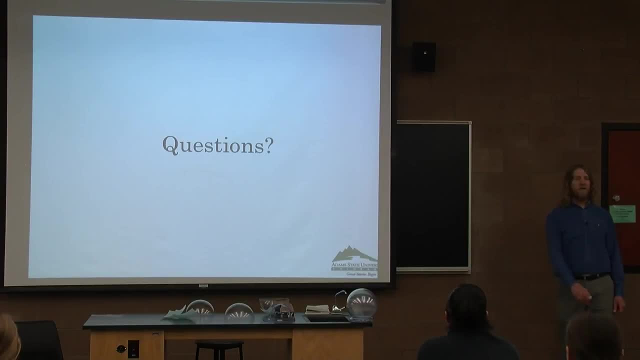 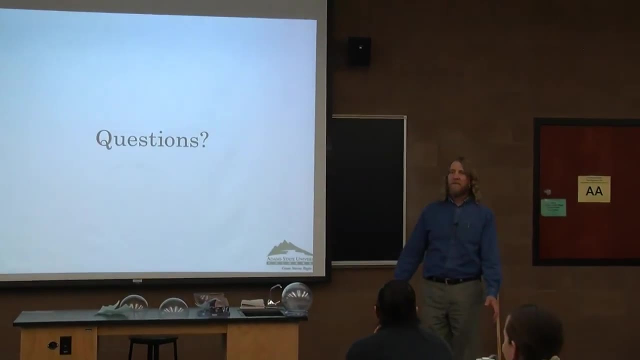 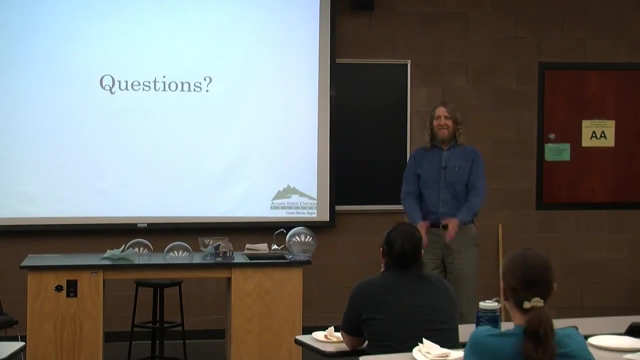 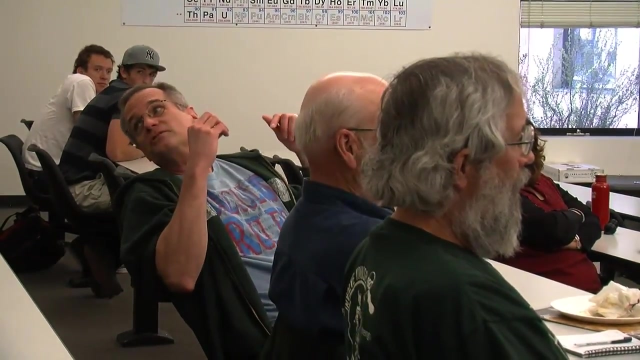 It's probably Euclidean. Any questions? Do I really have to answer that? Okay, Intellectual curiosity perhaps. Well, in astronomy we say if the universe is flat, then it's not going to collapse back. So if it's closed, it would be the elliptical geometry or spherical geometry and it would end up ending in a big crunch. 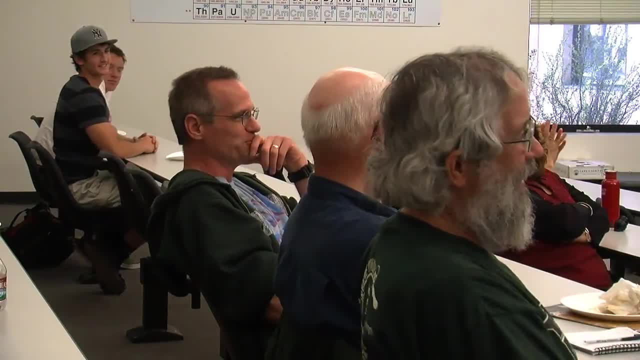 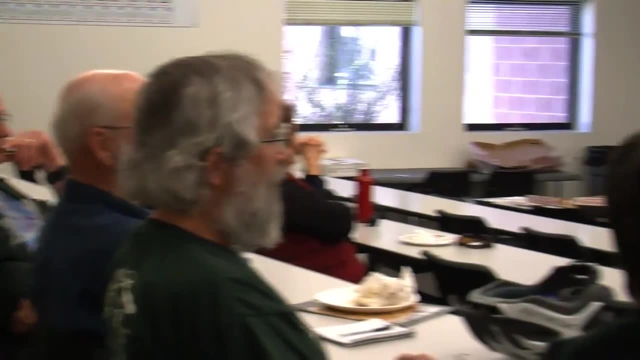 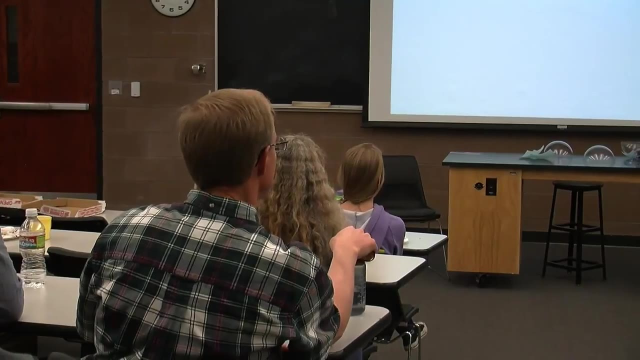 Yeah, So it does have. Okay, Yeah, Well, it seems to be flat. Yes, So I found it curious that you started off by saying we don't define points, lines and planes. Yeah, And then when you go to the spherical geometry, you have to define a line. 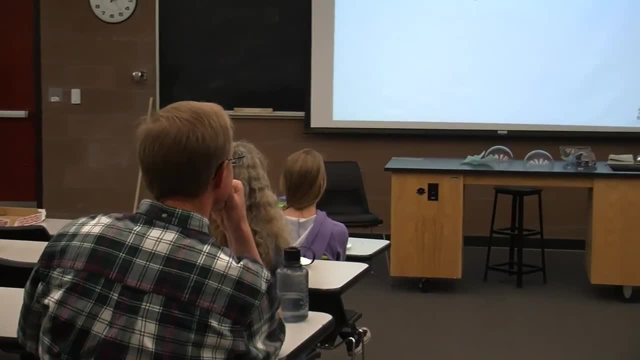 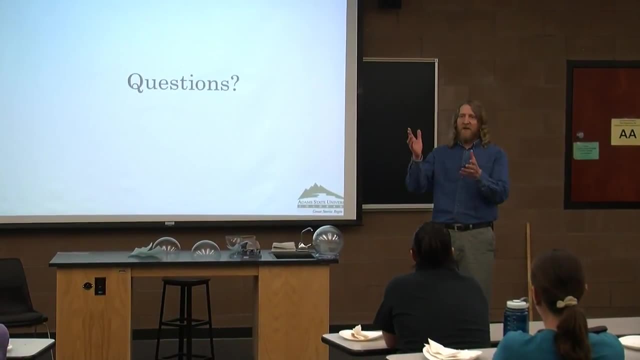 Well, because there you're talking about a specific model of that geometry. Okay, As opposed to just proving theorems in general, There is what's called neutral geometry. You can talk about these, These things that will apply in any geometry. 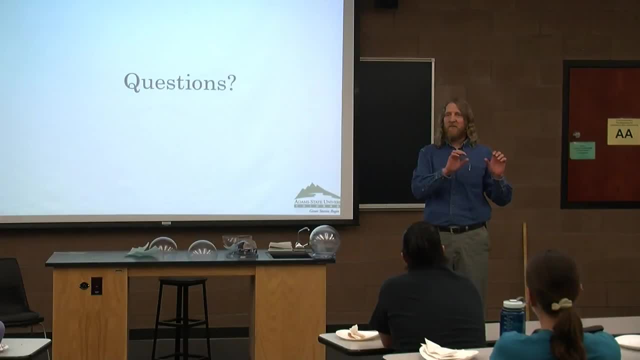 And when you're proving the theorems, you're trying to prove the most general case possible, And so, But in this specific model, yes, the lines are these things, And so, yeah, you do have to define them to narrow it down to a specific model. 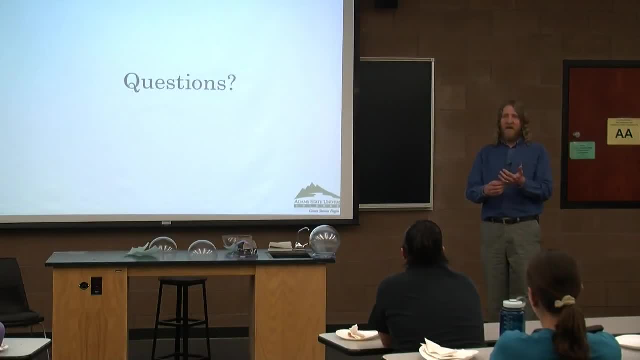 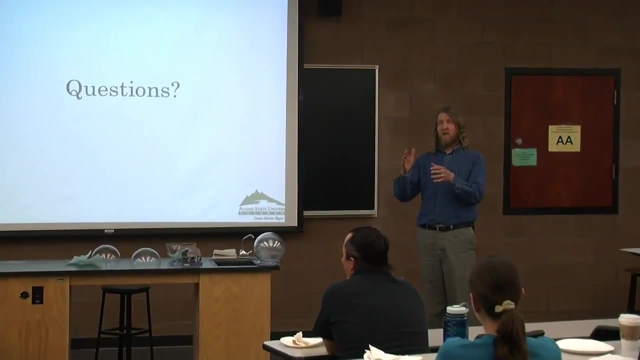 Because there are actually several models of each of these. I mean the hyperbolic. The Poincaré disk model is the most common. There's also what's called the Poincaré half-plane model, which is sort of like if you cut the disk and then smear it. 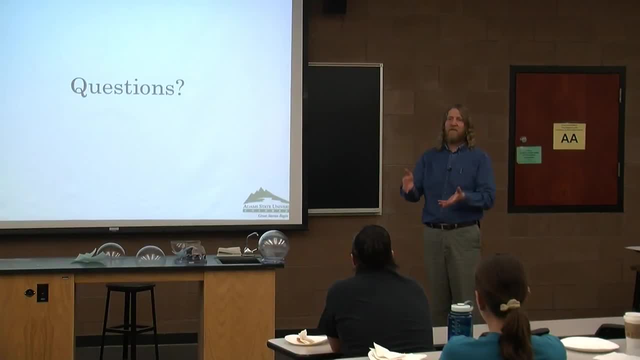 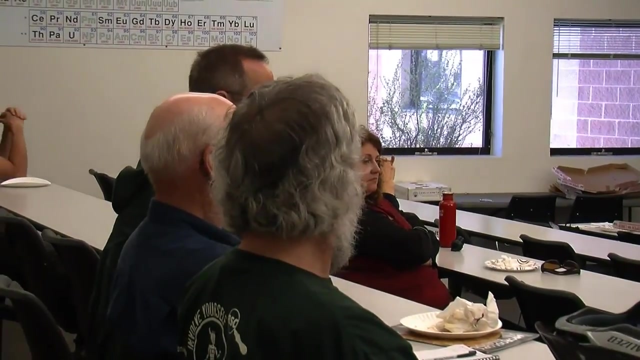 Yeah, Smeared it out like that. you can get a different model in which the lines look different, And so, yeah, you're right, We do have to define them to tailor it down to a specific model. Yeah, For the Poincaré disk model, is there a closed form function for distance between two points as a function of how far you are from the center? Yes, And I believe it's a function of the log of the distance from the edge. I believe I've seen it before, but I don't know it off the top of my head. But yes, there is. You can figure out the distance between two points in that geometry.